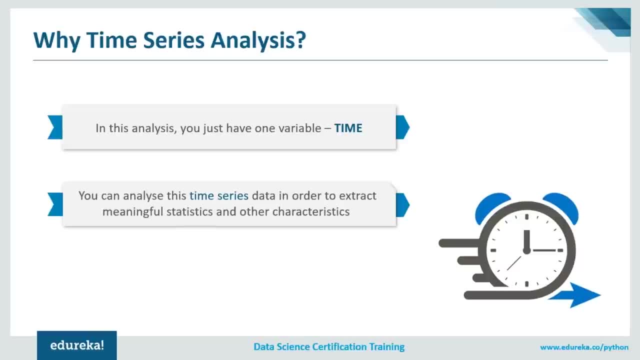 So let me explain you this with an example. Now let's take an example of a supervised learning. So under supervised learning we have linear regression or logistic. So there we have an independent variable and we have a dependent variable. So there, what we do? we deduce a function, or you can say a mapping function, of how one variable 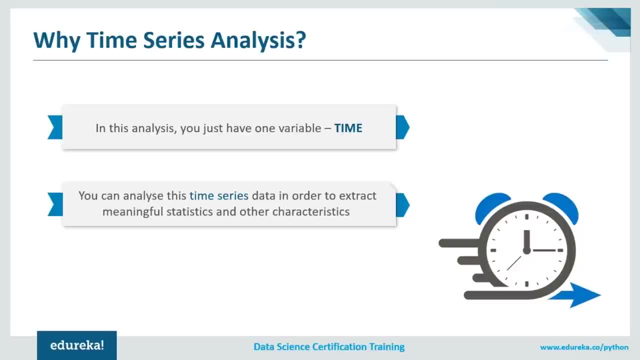 is related to another, and then we can go ahead with analysis part. But in time series analysis you just have one variable, that is time. So, for example, you own a coffee shop and it's quite a successful coffee shop in the town. So what do you do? you try to see how many number of cups of coffee you sell every month. 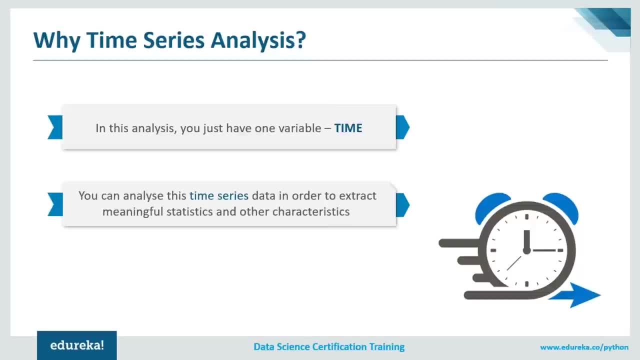 for that, what you will do, you add up all the sales of your coffee. Now let's say you started this coffee shop in the first month, That is, the January. So what you'll do, you'll record the data month wise, and then you will sum it up. 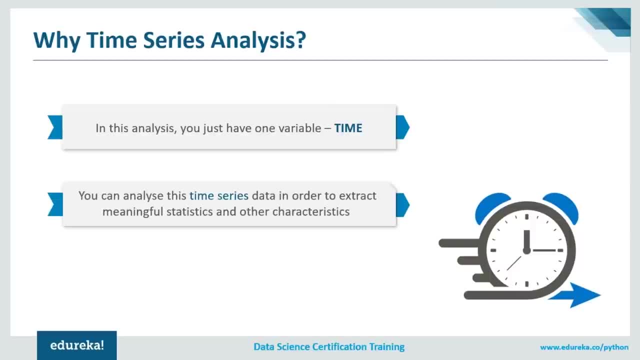 So you will have all the data till the present month. But what if you want to know the sales the next month or the next year? now imagine, guys, you just have one variable, that is sales, and you need to predict that variable in accordance with time. 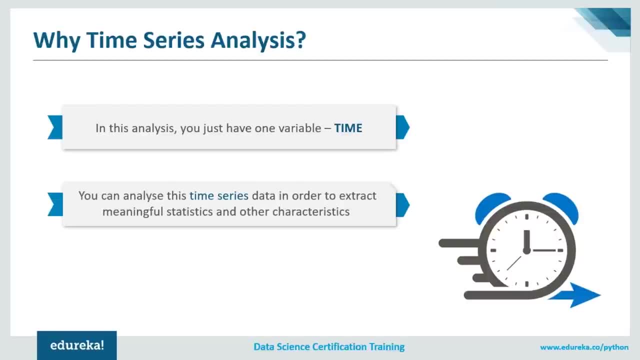 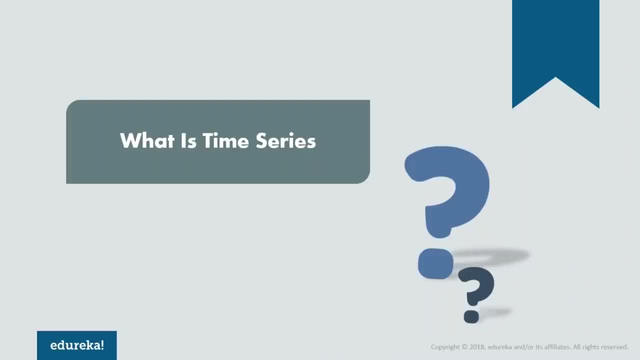 So in such cases, we'll just have time and you need to predict the other variable. You need time series analysis. Now we know why do we need time series analysis. Let's move ahead and understand what exactly time series is. So time series is a set of observations, or, you can say, data points. 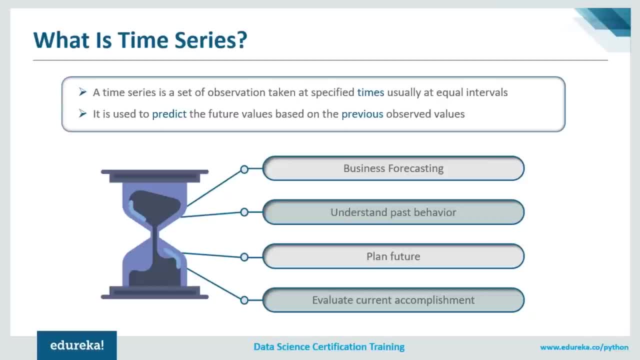 which are taken at a specified time. now over here at your x-axis You have the time and on the y-axis you have the magnitude of the data. So if you try to plot time series- plot on the x-axis- you will always get the time which is divided into equal intervals. 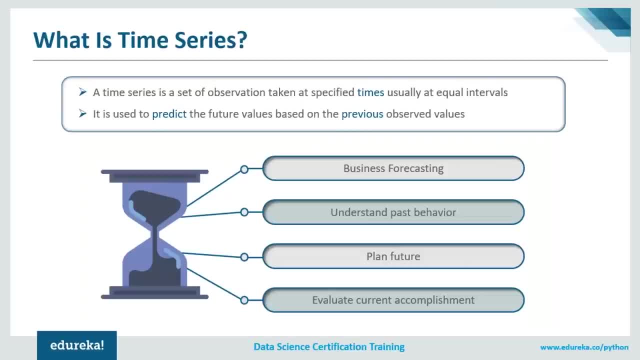 So cannot create a time series in one data point is at week level and other are different. They should be equal interval. Let's say a day, a week, a month, a year, a decade and a century. So that is the constant thing that a time series require. 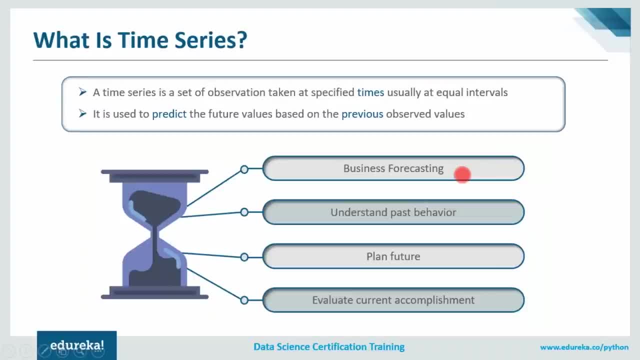 Now let us see the importance of time series analysis. Now, first and foremost is business forecasting, because your past defines what is going to happen in future. So let's say, you'll be seeing a lot of traders in the sense X who are trying to predict what will be the price of the stock market tomorrow. 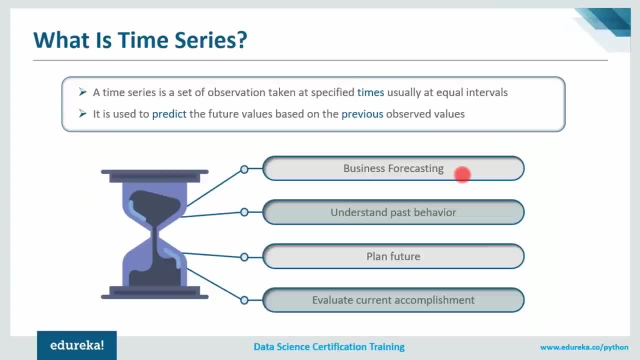 So that is nothing but a business Fasting. you also see a lot of retailers who tries to know how many number of goods they are going to sell the next day. So all of this can be achieved with time series analysis. Now, this is not just limited to one domain, like retail or Finance. 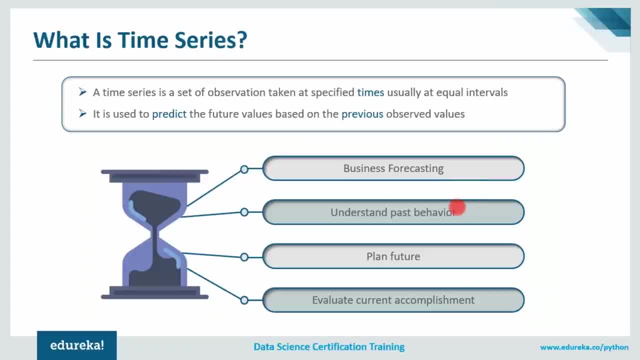 but it is applicable almost everywhere. Now it is also help us to analyze the past behavior. So here you can analyze in which month did the sales went up or when was the dip. so here you can easily understand your past data. So with every dip and a peak, there is a business reason attached to it. 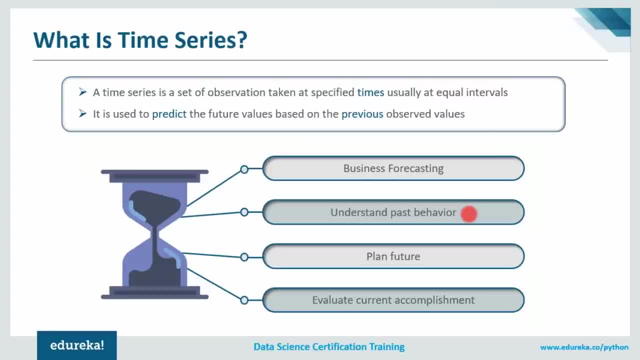 So you can understand this with respect to time. for example, some festival is there and you're selling chocolates, So your sales will increase during the festival, So you need to think about the seasonality part also. now, don't worry, guys will be having a complete discussion. 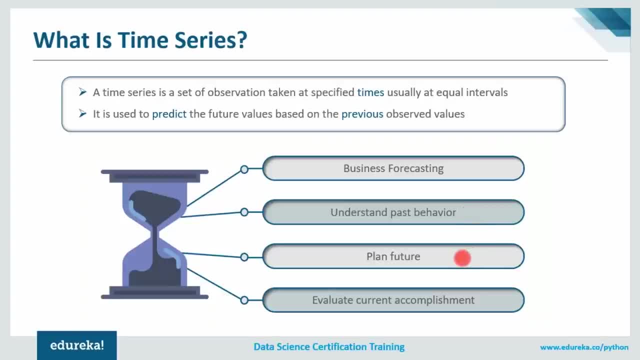 on seasonality as well. So now coming back, it also helps you to plan the future operations, so you can analyze the past and then you can forecast your future using this algorithm, that is, time series analysis. now, apart from all this, you can also evaluate current accomplishment. 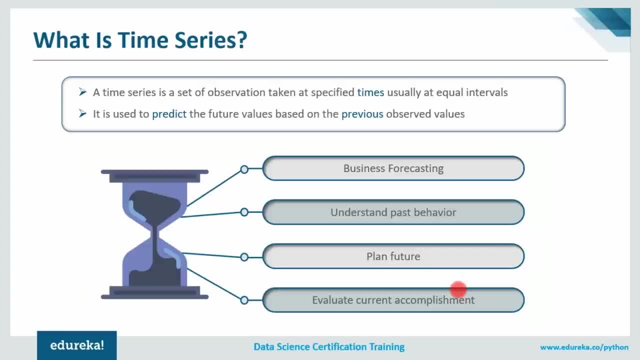 So this means you can determine which goals you have met in the current scenario. Let's say you have predicted, Okay, I'm going to sell around 100 chocolates in a day, but did you actually do that? So all of this can be analyzed using time series analysis. moving ahead, 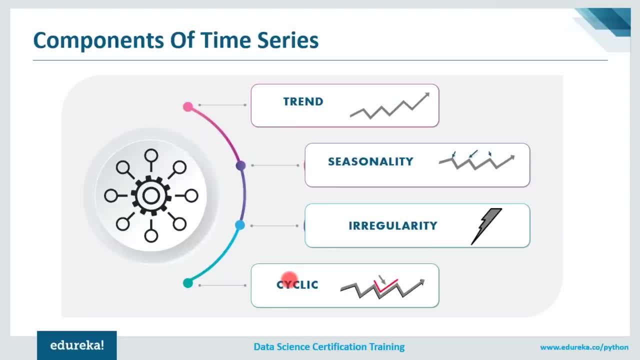 Let us see the different components of time series. Now, most of time series have trend, seasonality and irregularity associated with them, and some of them do have cyclic patterns also, but it is not compulsory that there has to be pattern present, So let us discuss each one of them in detail. 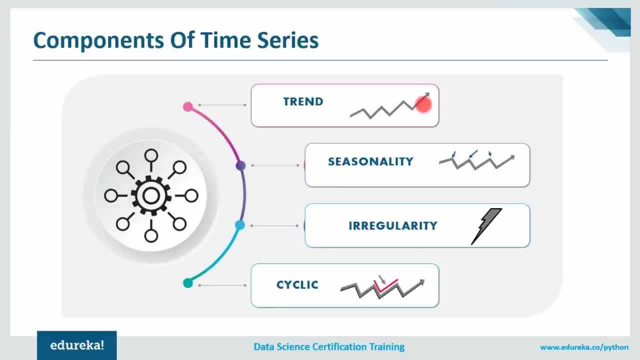 Now, the first is trend to trend is nothing but a movement to relatively higher or lower values over a long period of time. So when the time series analysis shows a general pattern that is upward, we call is an uptrend. also, if the trend exhibits a lower pattern that is down, we call it. 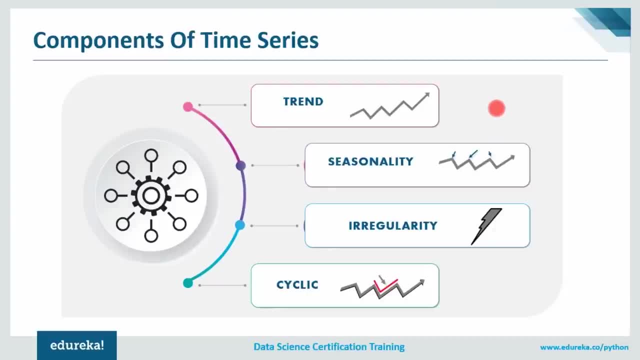 as a downtrend, and if there was no trend, we call it as a horizontal train, or you can say a stationary train. So now let me explain you better with an example. So there is a new township that has been constructed, Okay, and people are going to come and live over there. 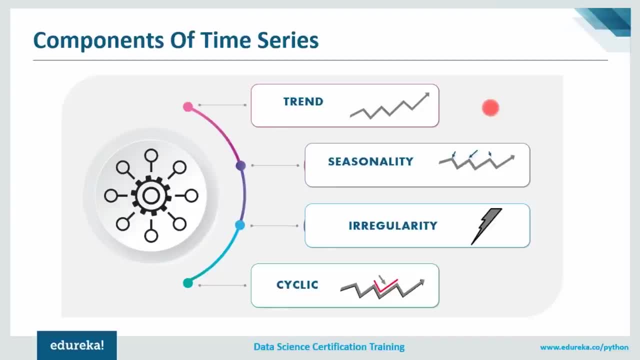 So what happens? a hardware guy comes up and opens up a shop there. So people will be coming up, will definitely buy stuff from there. Now, once all these houses are settled up or it's been occupied, the need of Hardware reduces, So the train may go down. 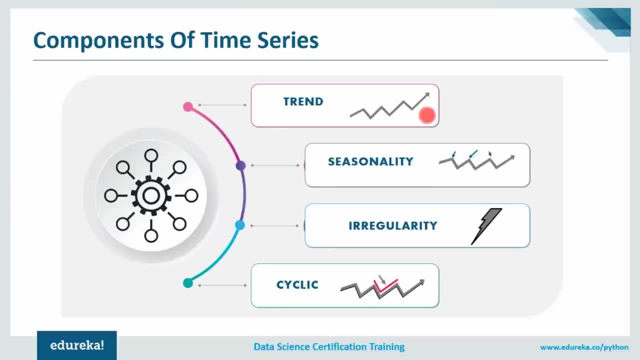 So let's say the sales were up in the first year and by another one year, or maybe in six months, It has gone down. So that is the train guys. So for some amount of time selling was high and then it got down. but this is not a pattern. 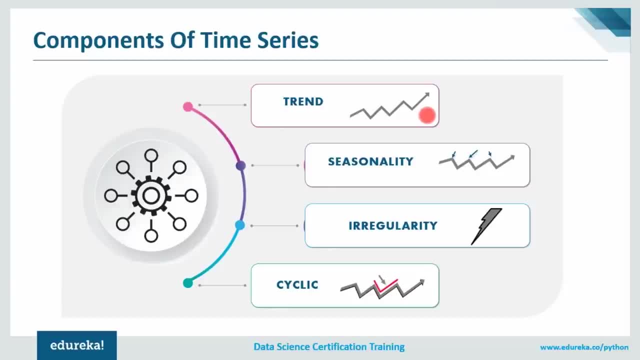 This is something that is happening year on year, but trend is something that happens for some time and then it disappears. Then we have seasonality. So here seasonality is basically upward or downward swings. but this is quite different. It's a repeating pattern within a fixed time period. 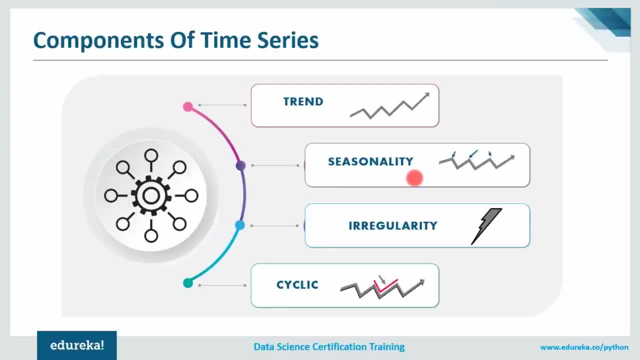 So, for example, Christmas happens every year on 25th December. Let's say you're on the business of chocolates, So every year on year, chocolates are served more and more in the last week of December. Now, this is because Christmas is there and you will be noticing this across the year, that is. 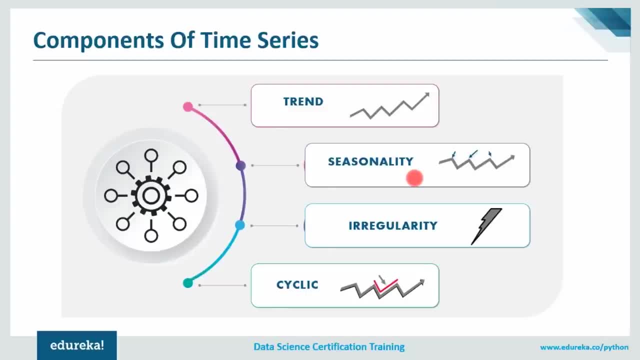 from past two years, four years, six years, 10 years and so on. So it's a repeating pattern, Then within a fixed time period, while in trend. that is not the case Now. let me take another example. Let's say ice cream this time. 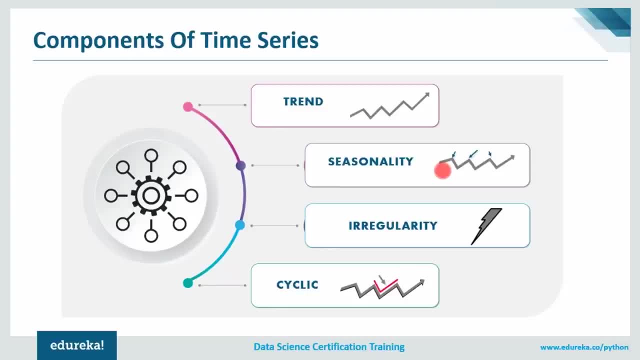 So ice cream sales will go comparatively higher in summers rather than in winter, So that is again a seasonality. then we have irregularity, or it is also called as noise, So these are erratic in nature, or you can say unsystematic. It is also called as residual. 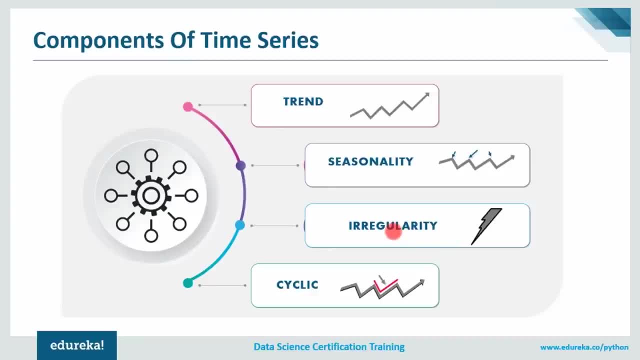 So this happens basically for short duration and is non-repeating. So here let me give you an example. So let's say there is a natural disaster, Let's say there is a flood in your town out of nowhere. in one year Now a lot of people are buying medicines. 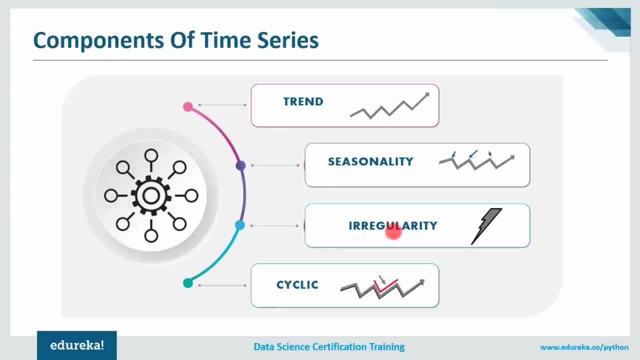 and ointment for relief. But after some time, when everything is settled up, the sales of those ointments have gone down. So this is something that no one could have predicted. It's going to happen erratically. You don't know how much number of sales are going to happen. 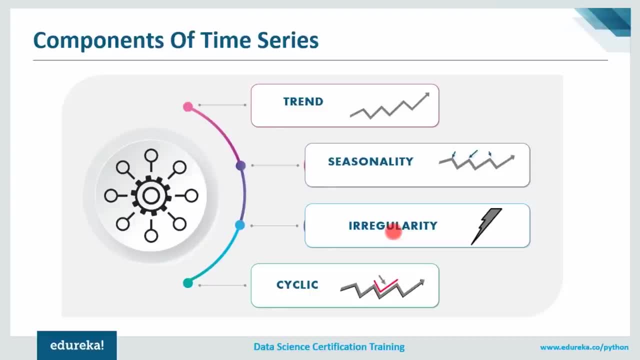 So you cannot force you about the event that the flood is happening. Okay, So this is some random variation, So this is what irregularity is now moving ahead. We have cyclic, So cyclic is basically repeating up and down movements, So this means you can go over more than a year. 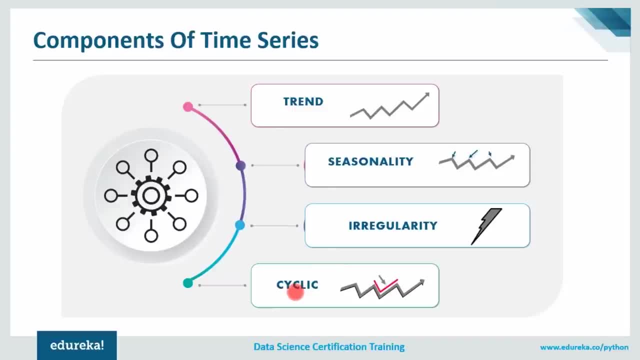 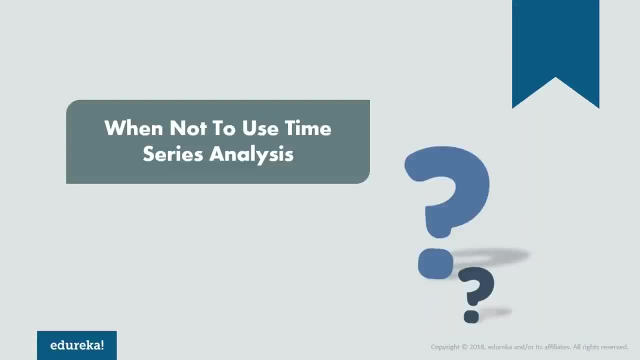 So they don't have a fixed pattern, so they can happen anytime. Let's say in two years, then fourth year, then maybe in six months. So they keep on repeating and they're much harder to predict. now, moving ahead, Let's discuss when not to apply time series analysis. 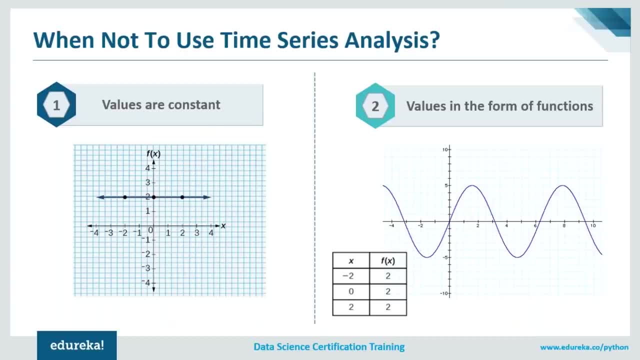 So first of all, you cannot see time series analysis when the values are constant. So let me take the same coffee example over here. So let's say the sales of number of coffee in the previous month is over 500, then this month also the sales number is almost. 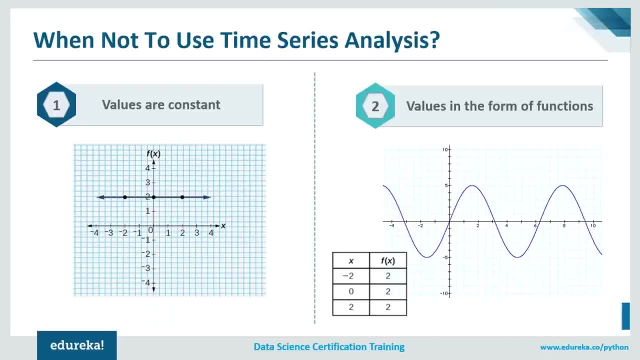 the same, that is, 500.. I wanted to predict the number of sales in the next month. now, in such cases with the values are constant, as in an R case, the number of sales of 500 in the previous month and then in this month also, we have the same number. 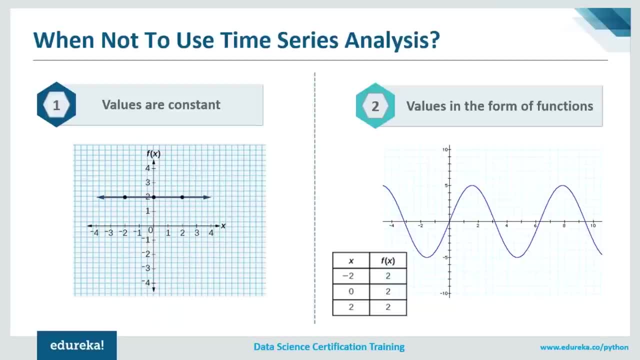 and now we want to predict it for the next month. So in such cases where the values are constant, time series cannot be applied. Similarly, if you have values in the form of functions- let's say you have sine of X or cos of X- 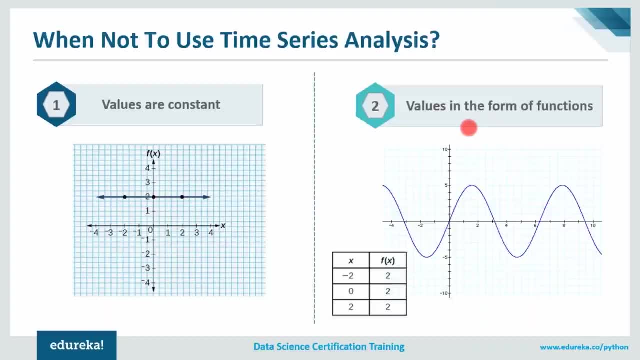 So, for example, in this case you have X value and you can get the value by just putting it in the function. So there is no point of applying time series analysis, where you can calculate the values by just using a function. now you can apply time series to these as well. 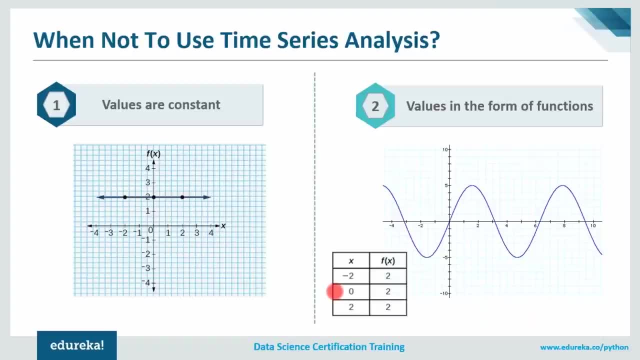 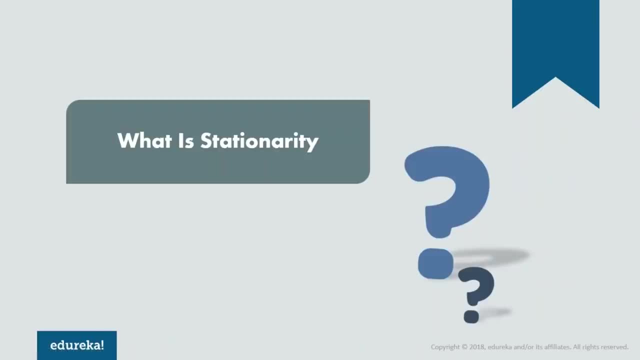 But again, there is no point of applying it if you have a formula before that or the values are just constant. So these are the cases when you should not apply time series. moving ahead, Let us see What is stationarity. So no matter what guys, how much you try to avoid the stationarity, 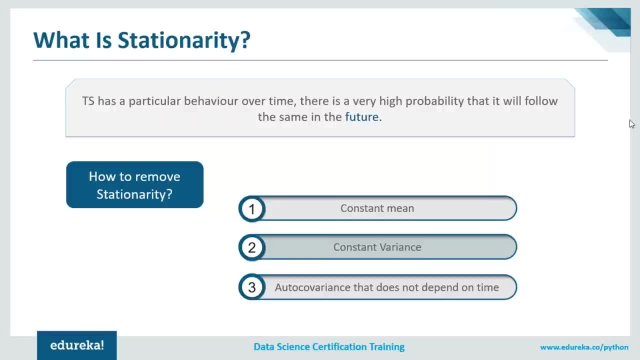 part. It will always be there in time series. So here, time series requires the data to be stationary. So any kind of statistical model that you apply on time series, the data should be stationary. So let's understand what exactly it is. Now most of the models work on the assumption that time series 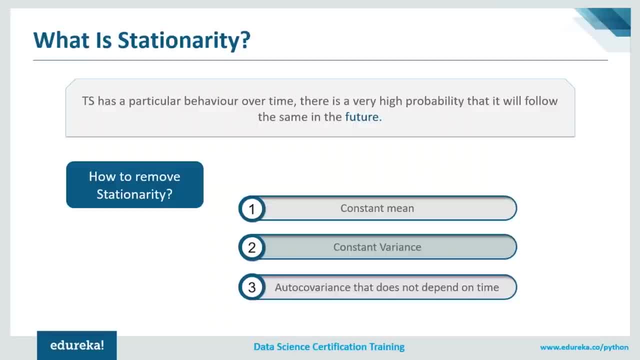 is stationary Now. if the time series has a particular behavior over time, there is a very high probability that it will have that it will follow the same in the future. Also, the theories and formulas that are related to stationary series are more mature and easier to implement as compared to a non-stationary. 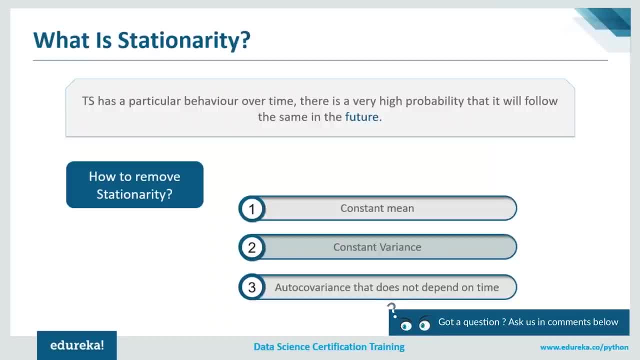 series. Now, there are two major reasons behind the non-stationary of a time series. So first is trend, which is basically the varying mean over time. Secondly, we have seasonality, So this is the variation of a specific time frames. but did you guys get the answer to this question? 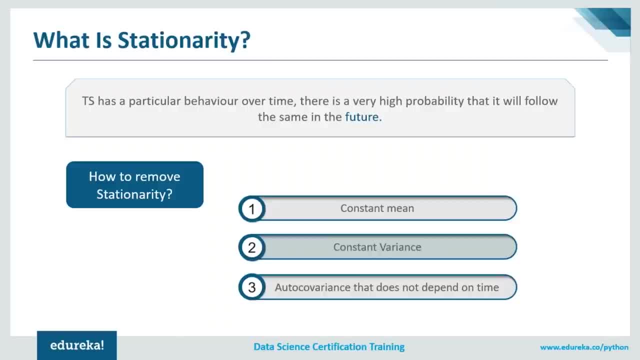 What exactly is stationary, or how exactly is stationality is defined. So stationarity basically has a very strict criteria. The first one is it should have a constant mean. now, here the mean should be constant According to the time. Secondly, we have constant variance. 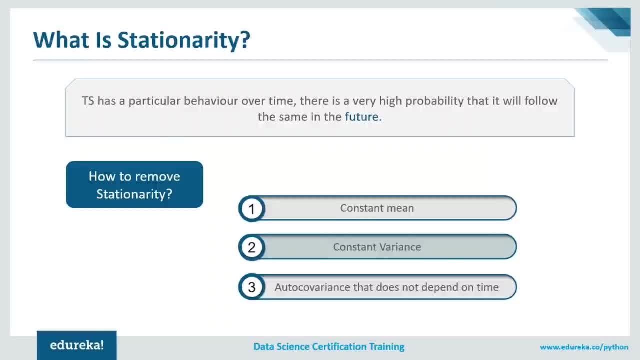 So again, variance should be equal at different time intervals and thirdly, we have auto covariance that does not depend on time. So for those of you who don't know what mean is, I'll not go into the details, but I'll just explain you in a nutshell. 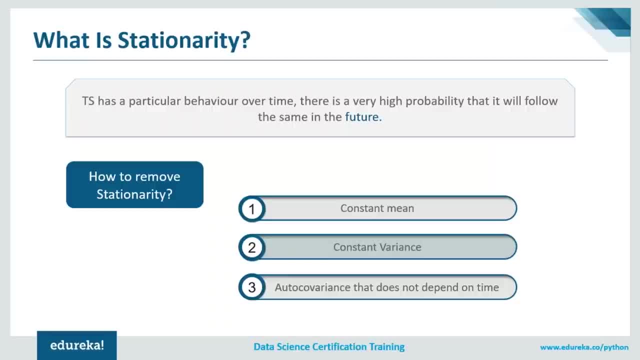 So mean is basically the average. then variance is just the distance from the mean. so each points distance from the mean should be equal, and then we have auto covariance. that should not depend on time, or it should be equal as well. For example, let's say you're standing at time. 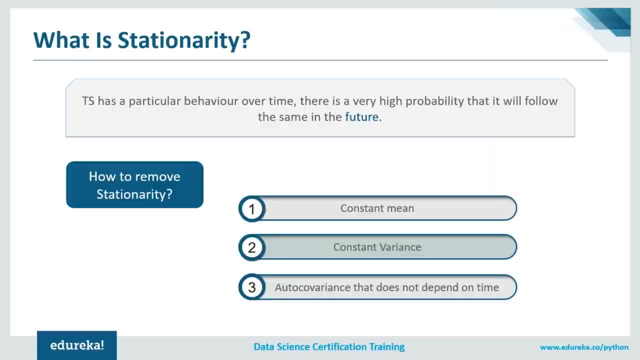 Okay, and your previous time period was t-1 or t-2.. Let's say there are previous two time periods. So the values at t-2 or t-1 P, they should not have any kind of correlation between them, which is basically dependent on your time period. 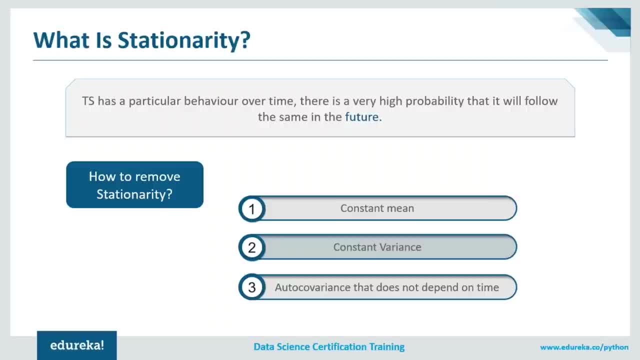 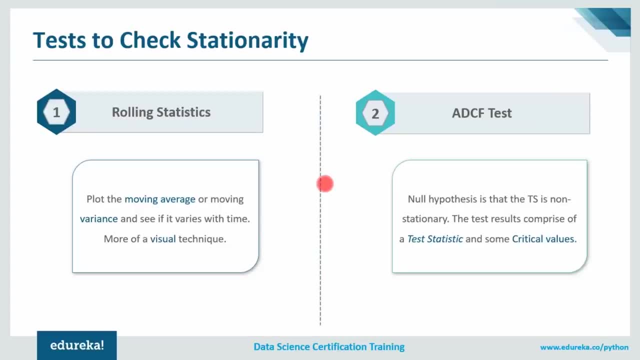 So that is nothing but auto covariance. So when these three conditions are met, then we can say at series is stationary, and then we can apply time series analysis over it. now to check the stationarity in Python We have two popular test now. first is ruling statistics. 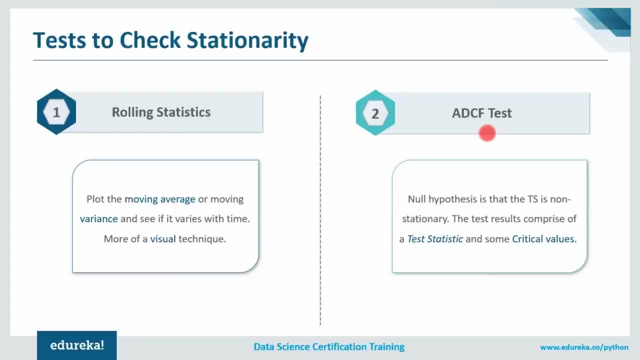 and the second is a DCF, or you can say augmented Dickey fuller test. now in ruling statistics We can plot the moving average, or you can say moving variance and see if it varies with time. now by moving average of variance I mean that any instance T will take the average or variance. 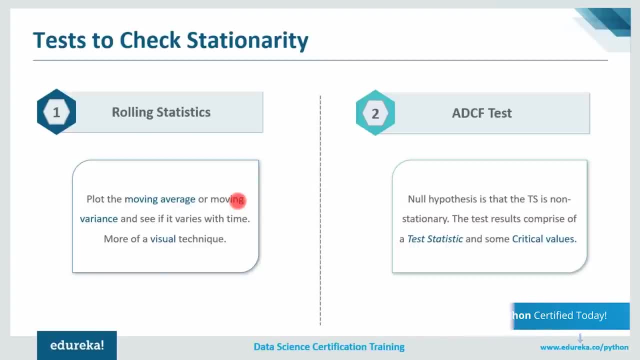 of time window, Let's say, if you want to know for the last year, that is, for last 12 months or anything. and also, guys is more of a visual technique, so you cannot deploy this kind of stuff on production, but it is quite useful for the POC purpose. 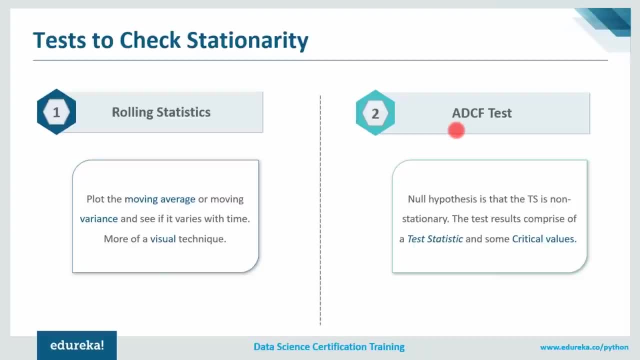 Then we have a DCF. You can say augmented Dickey fuller test in the world of data science. So Dickey fuller test, which is another statistical test for checking stationarity. now here you have the null hypothesis, which is time series is non-stationary. 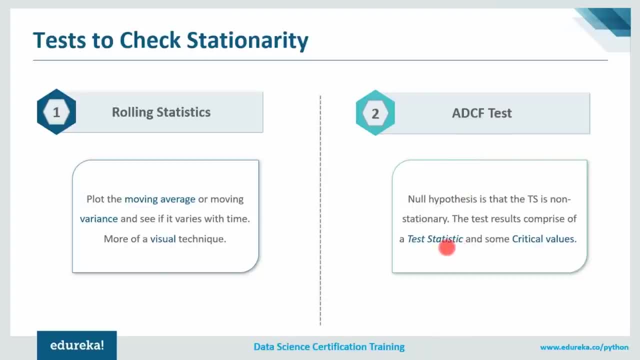 and once you perform this test, you'll get a result which comprises of a test statistic and some critical values for different confidence level. now here it is said that if the test statistic is less than the critical value, we can reject the null hypothesis and say that the series is stationary. 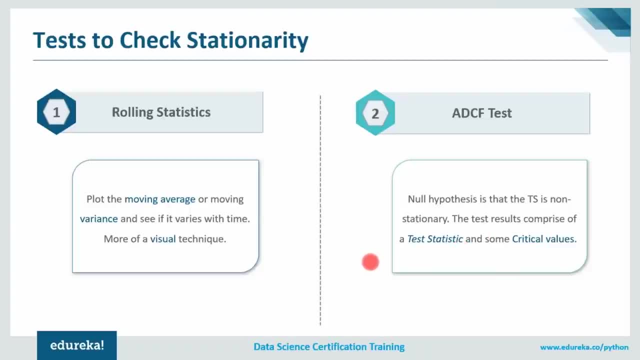 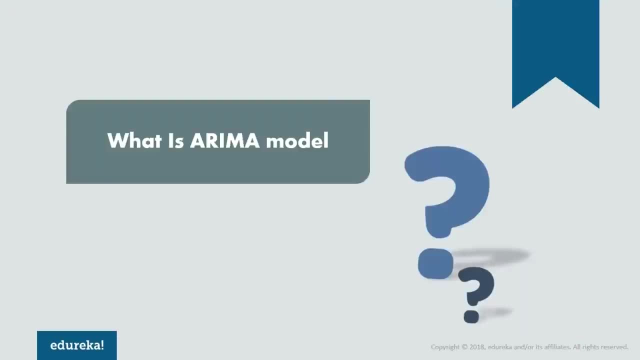 So don't worry, guys, I'll be explaining this again when we go to a demo part, but I hope you guys are clear with what exactly stationary and how we can check the stationarity. All right, So now let me just move on to my next topic. 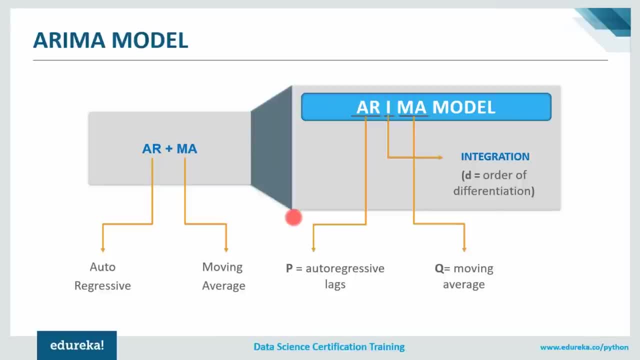 So now we'll discuss what exactly is Arima model? now, Arima is one of the best model to work with time series data. So this is basically the combination of two models, that is, AR plus ma, and it's quite powerful guys. So once you combine both of these model, you get the Arima. 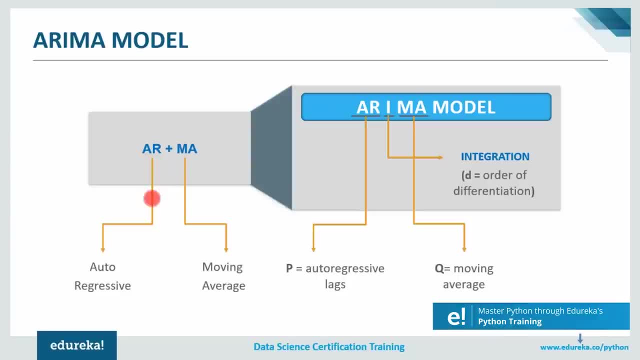 model. now, your AR model stands for autoregressive part and ma model stands for moving Average. so AR is a separate model, ma is a separate model and what binds it together is the integration part that is indicated by I. so AR is nothing but the correlation between the previous time period. 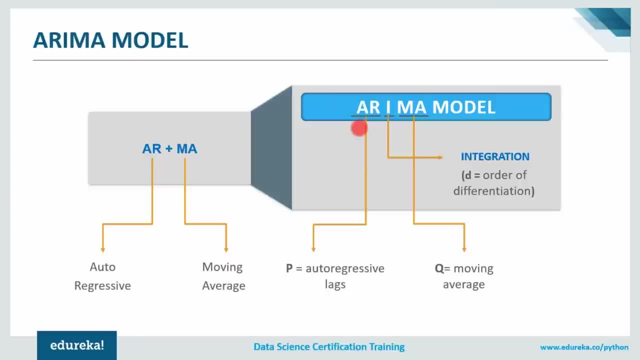 to the current. So what does this mean? now, Let's take this into consideration: that you are standing at a time period, T, and there are previous time periods like T minus 1, T minus 2, T minus 3. now, if you find any correlation, 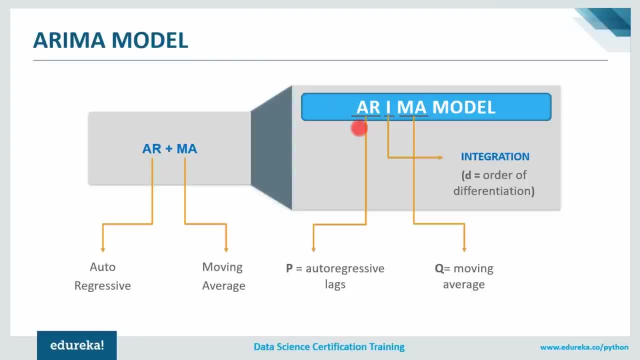 between T minus 3 and T. that is nothing but the autoregressive part. So, as I told you earlier that there is always some kind of noise or irregularity attached in a time series, So we need to figure out that noise. In fact, we need to average that out now whenever we try. 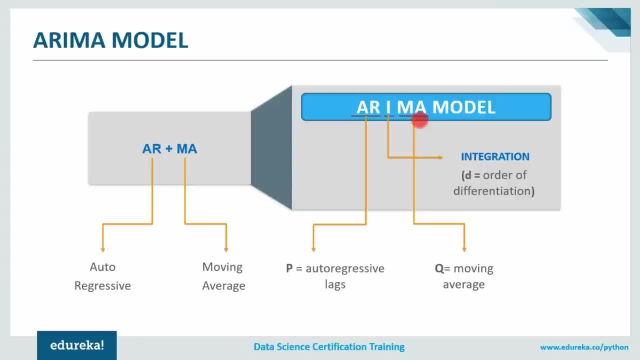 to average it out, the crust and traps that are present in that noise smoothen out and we can have average forecast of that noise. You can actually never predict when a next customer is going to come in and buy hundred items at once, So we try to soothe it up by taking its average now. 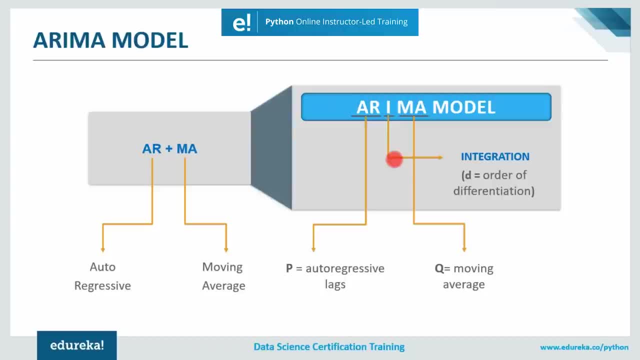 Arima model has three parameters. It has P, it has Q and has D. So P basically refers to your autoregressive lags, then Q stands for moving average and D is the order of differentiation. So we have each parameter for each of the models. 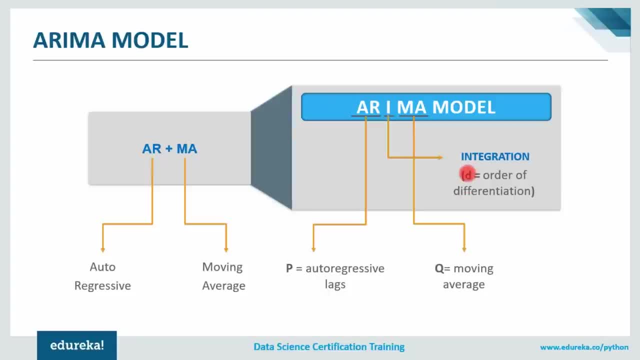 So if we take the integration by just one order, then the value of D would be one. if we differentiate it in the order of two, then we have the value D equals to 2.. So that is how we can predict these values: P, Q and D. 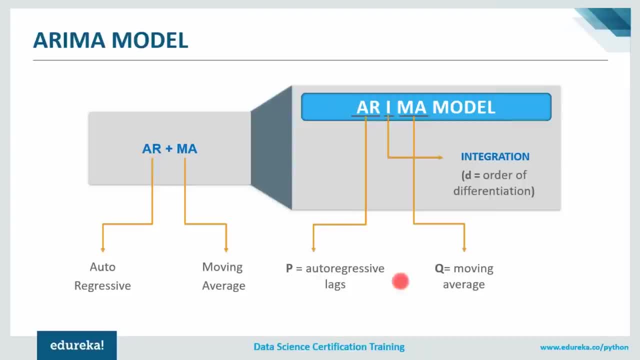 and each of them has a different method to it. So if you want to predict the value of P, you will be using an PSEF graph. that is nothing but a partial autocorrelation graph. then to predict Q value, We need to plot ACF plot. that is autocorrelation plot. 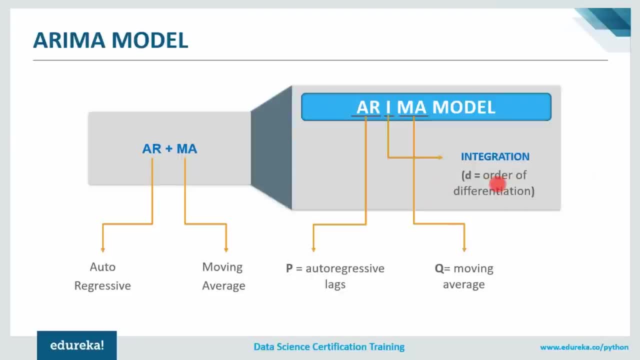 and D. I have already told you, to make data stationary We use some kind of differentiation, So the order of differentiation defines the value D. So I guess enough of theory part. So now let's quickly jump on to the demo and let's see how you can implement all of these things. 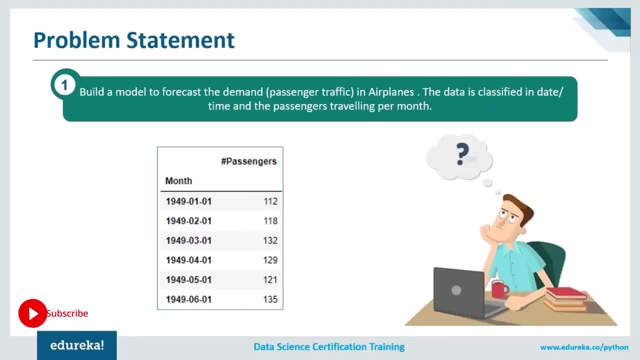 So now we'll have a look to a demo and we'll focus the future. So here we have a problem statement with is a line which has the data of passengers across months. So here what you need to do: you need to build a forecast to determine how many number of passengers are going. 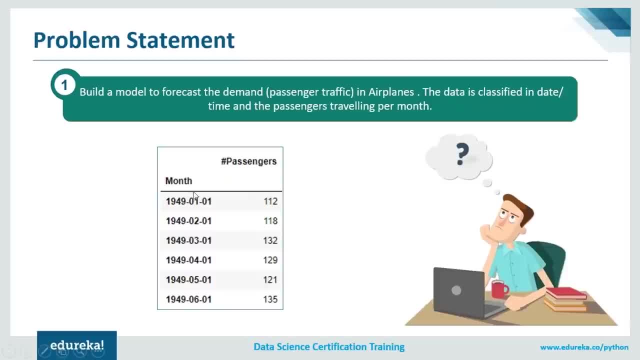 to abort these Airlines at the month level in the future. So here we have month, or you can say dates. So here we have dates from 1949 to 1960 and we have the number of passengers traveling per month. So now we have this kind of data. 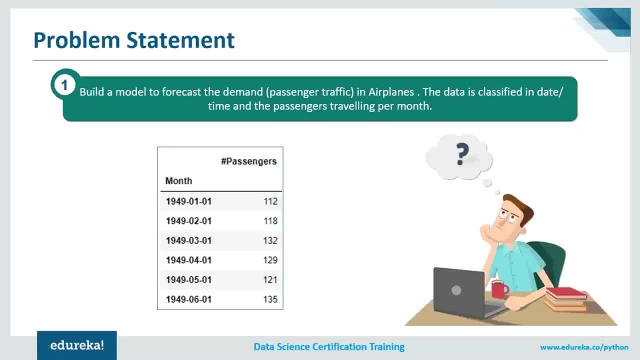 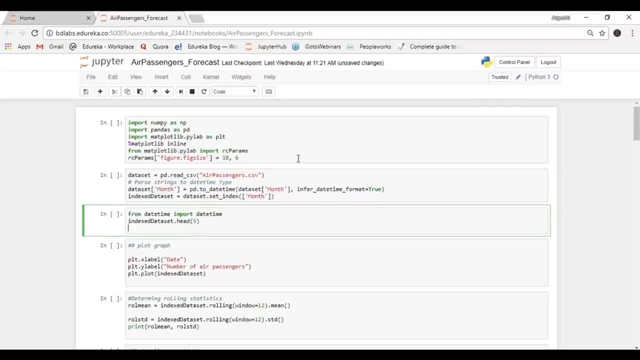 and we need to analyze what will be the number of passengers if we have to predict it for next 10 years. So now let me just go to my Jupiter notebook and let us see how my predictions look like. So guys, my Jupiter notebook, million, I have the code. 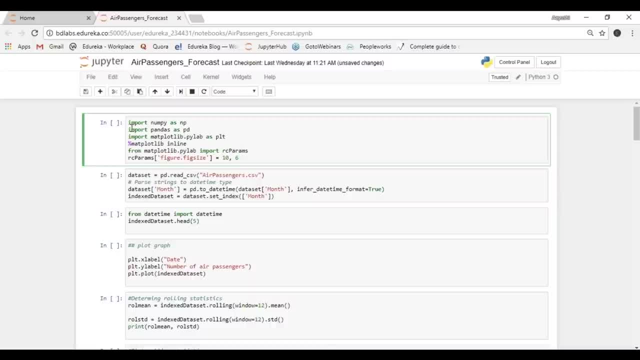 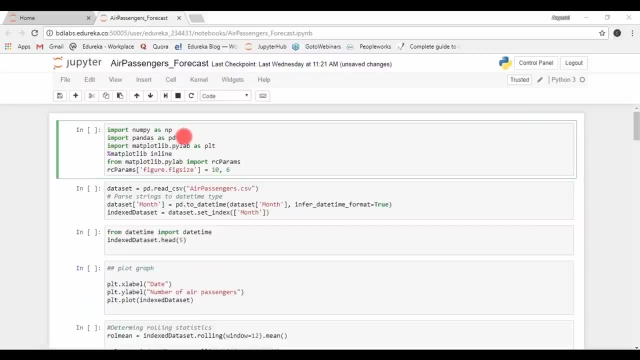 and we'll be implementing all the things that we have discussed till now. So first of all we'll be importing all the necessary libraries. So here we have imported numpy, then we have imported pandas for data analysis part and you can say data processing. then we have imported matplotlib. 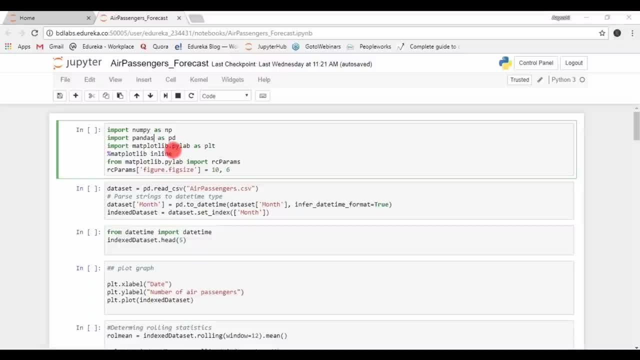 for data visualization, creating plots and all those things. then order to implement matplotlib. We have also written percentage matplotlib in line for Jupiter notebook, So not get a particular plot open in a new window. Everything will be there in your Jupiter notebook itself. And then I have just defined the size. 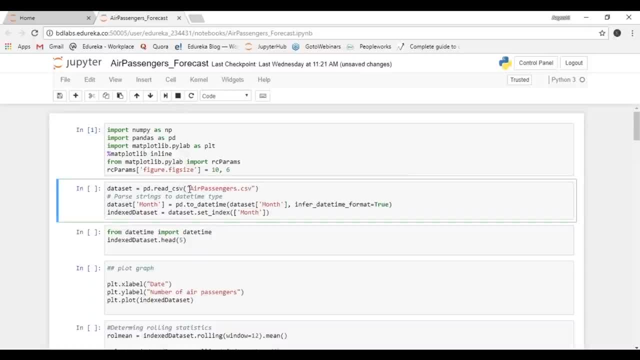 So now let me just run this. Next what I've done. I have imported my air passengers data using pandas, So we have a function of read CSV in Panda that is represented with PD. So we have substituted this in a variable data set. and then what we have done: 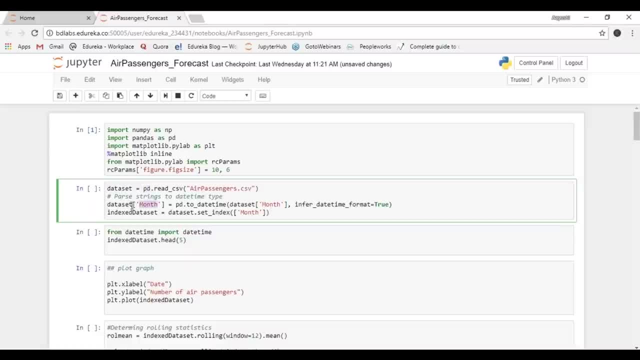 We have just passed those strings in a date time format, So here we have set our data month wise. So using pandas we have a function to date time. So over here you can specify a month and then you can just set this as your index. 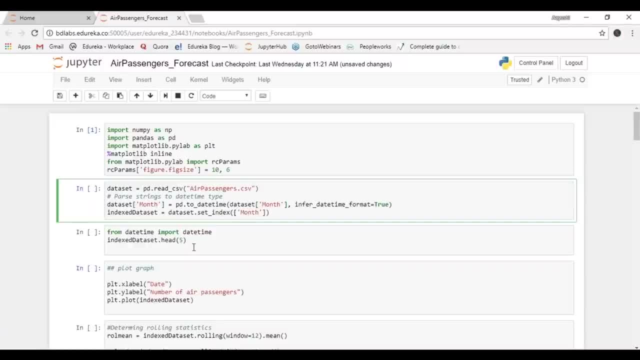 So here you have index variable as month. next, what I have done: I have imported date time and then I have just printed the top five values. So now let me just run this. This is how my data looks like. I have month as my index. 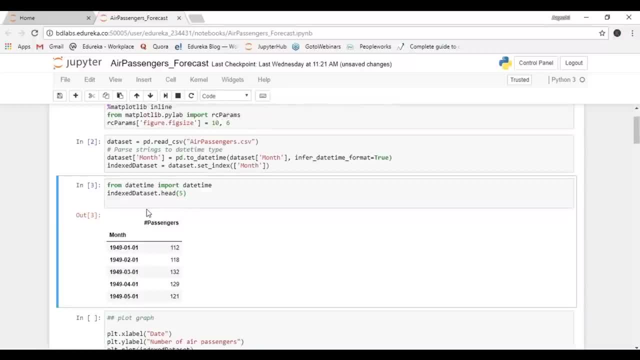 and then I have number of passengers as my second column. So this data I've already showed you in the presentation, where I have the data from 1949 until 1960.. So I have just printed the head of it, So now let me just print the tail. 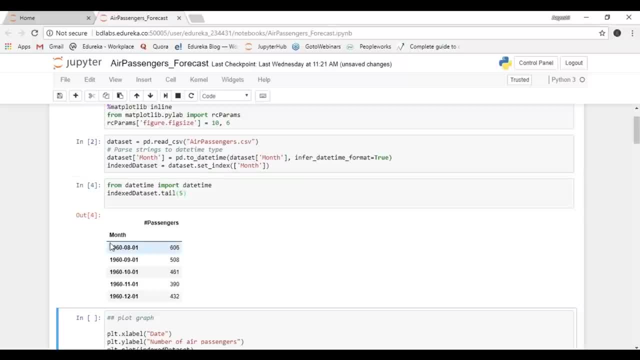 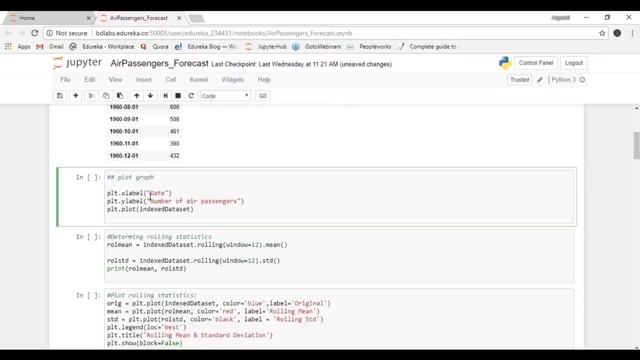 So let's say, I want to know the last five data entries. So here we have data till 1960 and we have the number of passengers next. what we have done, We have simply plotted a graph between them. So, guys in time series. 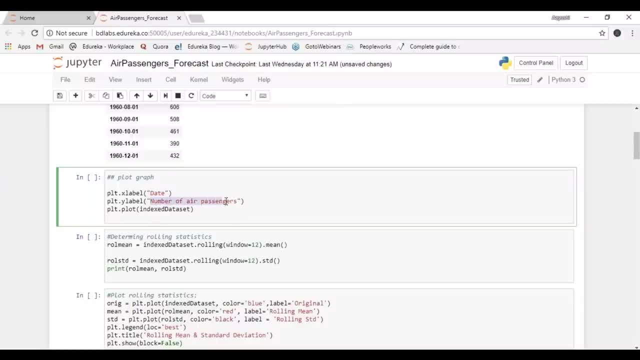 we have date and we have another variable. So here my other variable is number of air passengers. So here we have date on my x-axis and number of passengers on my y-axis, and then we have simply plot that graph. So now let me just run this. 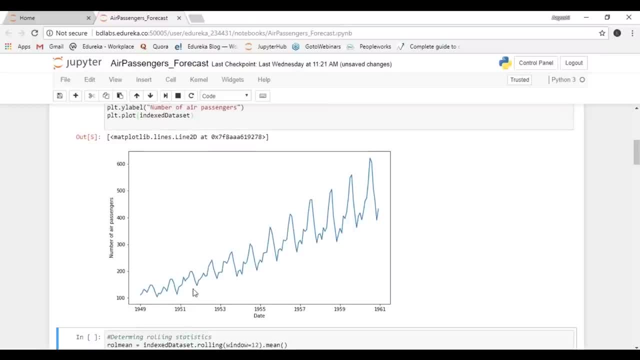 So this is how your data look like. So here, if you notice, you have a trend. So your next step is to check the stationarity. So I'll give you 10 second, guys, and think whether this data is stationary or not. So just think and give me a reply. 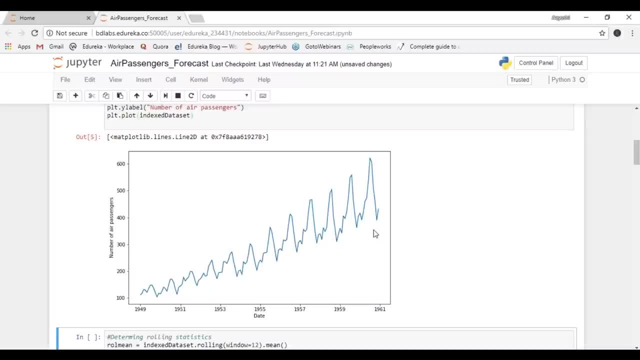 whether this data is stationary or not, Right, Shivani? So this data is non-stationary. So here you can see, the trend is going up. So let's say, if you want to calculate the mean at 1951.. So here your mean will lie somewhat over here. 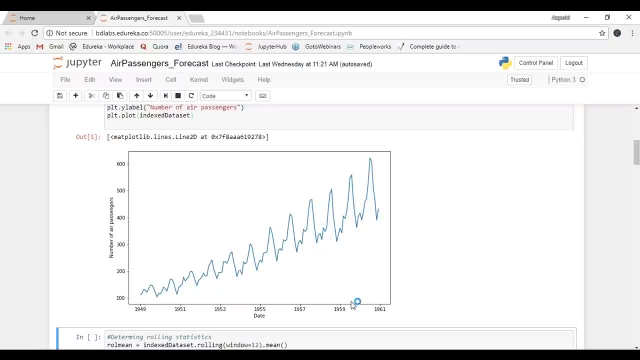 and let's, if you want, to calculate the mean of this year, that is 1960.. So here your mean will be somewhere here. So here you can see that you have a upward trend and the mean is not constant. So this tells me your data is not stationary. 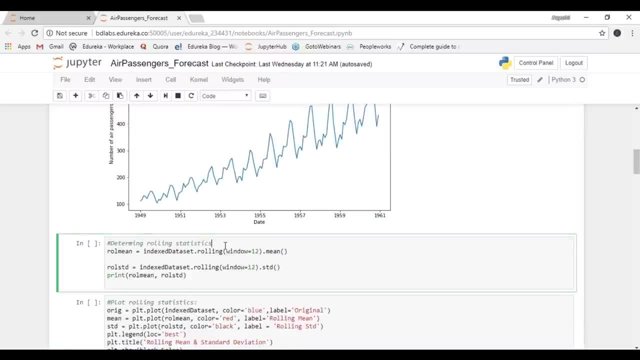 So now I have told you guys that there are two tests, which basically helps you in checking the stationarity of the data. So here we have rolling statistics as well as we have ADCF, So let's go through each one of them. So here we'll be, first going to the rolling statistics. 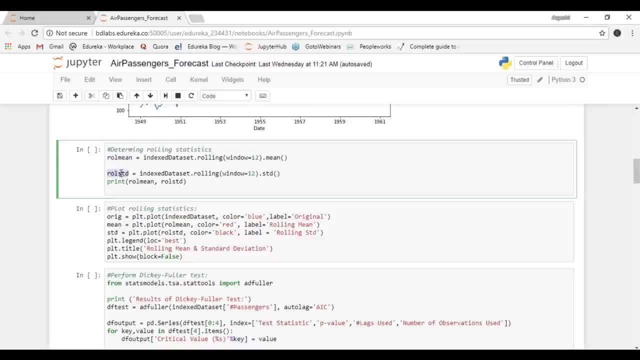 So here we have rolling mean and we have rolling standard deviation. So here, as you can see, we have a window of 12. that is nothing but the window of 12 months. So let's say we have Jan of 1949 and you place the value of Jan 1950 with the value of 1949. 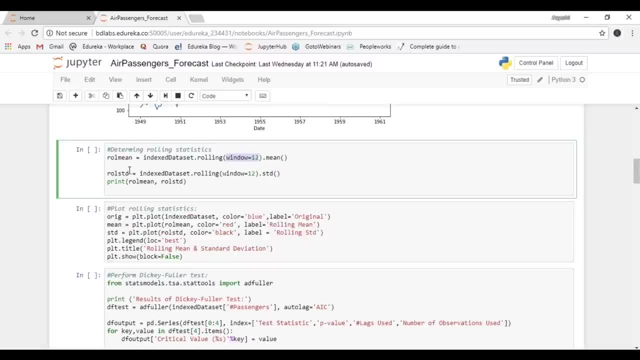 So this gives you the rolling mean at yearly level and you have to do the same with the standard deviation as well. So in Python to calculate mean and standard deviation, you have a function, dot mean, and you have dot STD, So this will automatically calculate mean. 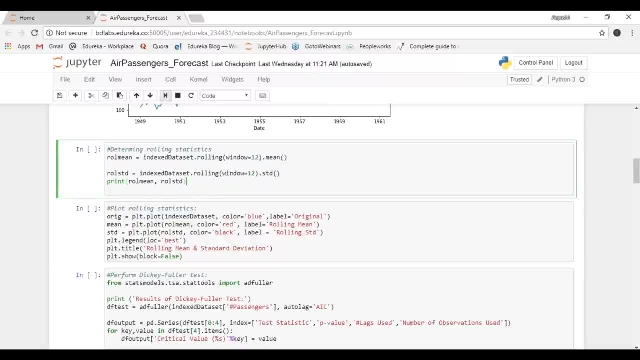 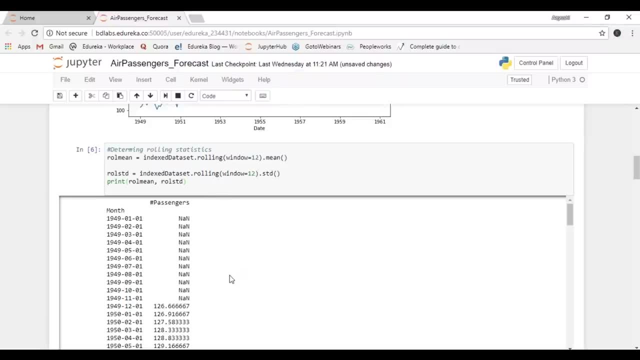 and standard deviation. So now let me just run this. So here, if you notice, your first 11 rows is nan. that is not a number. now, this is because we have calculated all the averages of these 11 and given over here, and similarly you can do the same for the next ones. next, 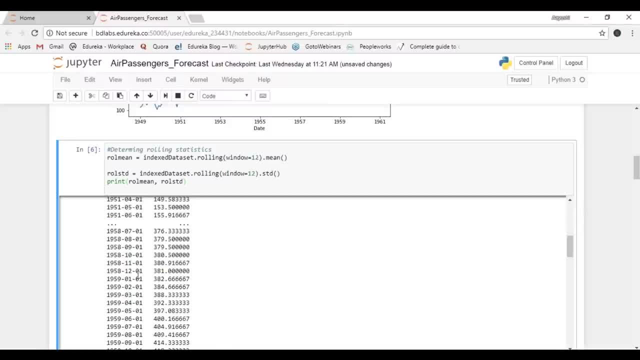 if you just crawl a little bit you see it's a long data set and you have the same result for standard deviation as well. So it's the same procedure, guys. average has been calculated and then just given out. So here must be having a question by only 11 values are nan. 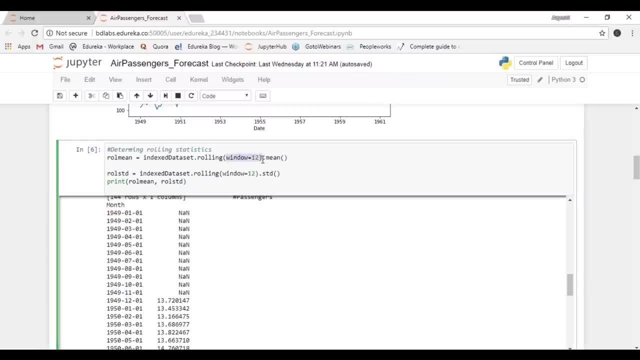 So over here we have just given a window of 12.. Let's have given a window at daily basis, or you have date at a day level. Then your window size would be 365.. So here my data is at monthly levels, So the focus will be on monthly only now. 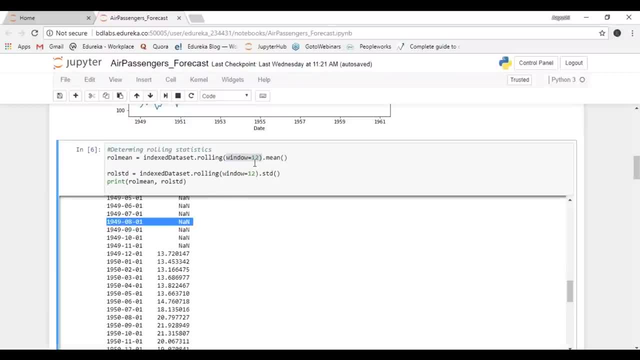 Similarly, if you have data at day level, then probably a window can be 365.. So I hope you get the reason why I am giving the wind as 12 and why we are calculating the mean and standard deviation. Then what we have done, we have simply plotted. 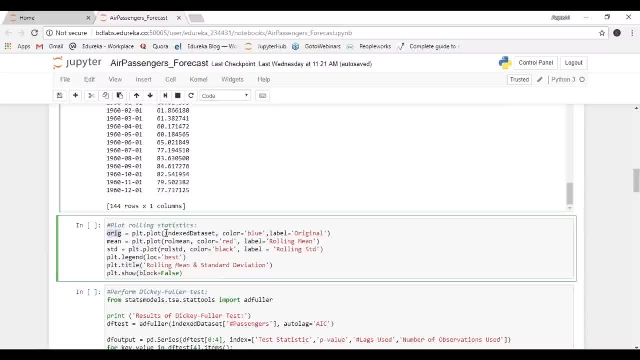 this rolling statistics bar. So here we have the original data, which is just plotted by the color blue. Then we have the mean data. So here we have just plotted the mean for what we have just calculated above, and then we have given the color red to it. 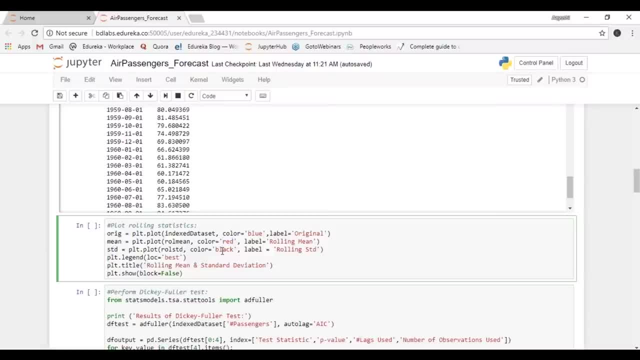 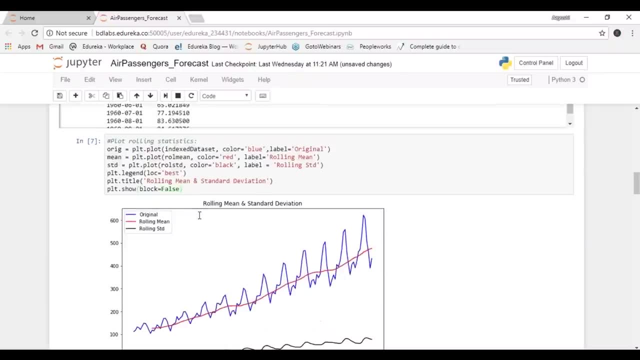 Similarly, we have plotted the same for standard deviation, and we have given a color black to it. after that, We have just given a legend, we have given a title to it, And now let me just run this code for you. So over here you can see, we have a plot somewhat like this. 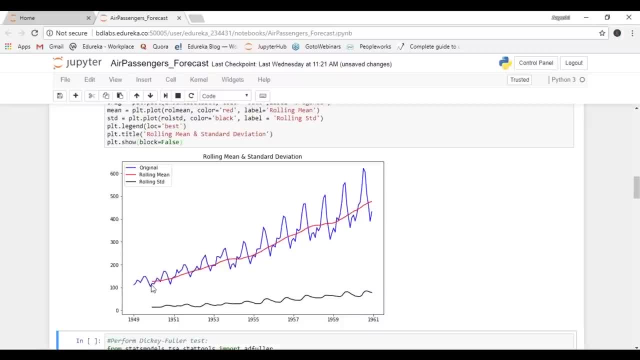 So, guys, blue line is my original data and, as you can see, I have my mean in red and I have a rolling standard deviation in black color. So over here you can conclude that your mean and even your standard deviation is not constant, So your data is not stationary. 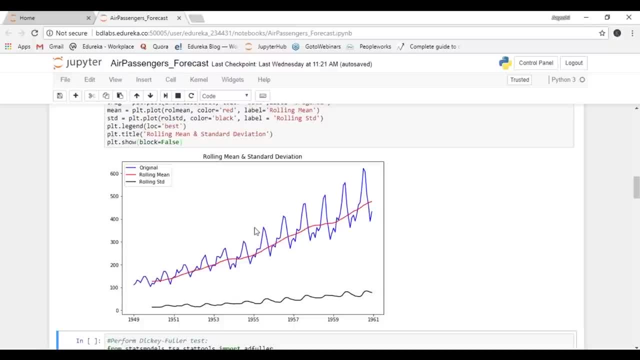 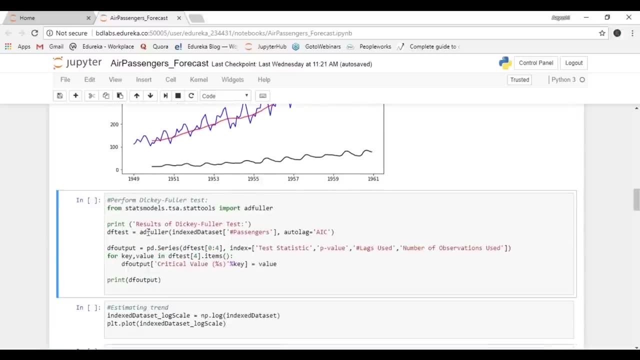 So, guys, this is my rolling statistics method is again a visual technique. So here we have already concluded that this is not a stationary data set. Now let me perform the key for the test as well. So to perform the key for the test in Python. 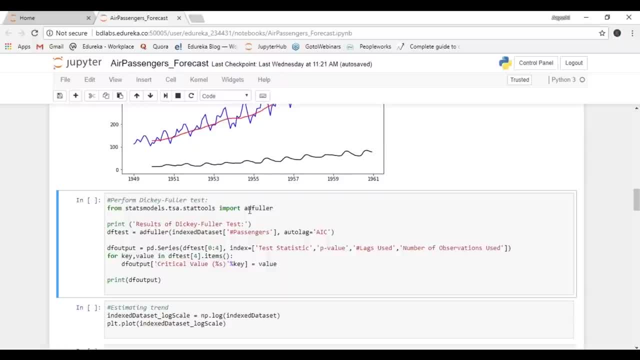 you have to import from stats model to TSA stat tools. import a D fuller. Now this is the function which has been provided in the key fuller test. So here I have a function that is a D filler. I have passed the data set into it. 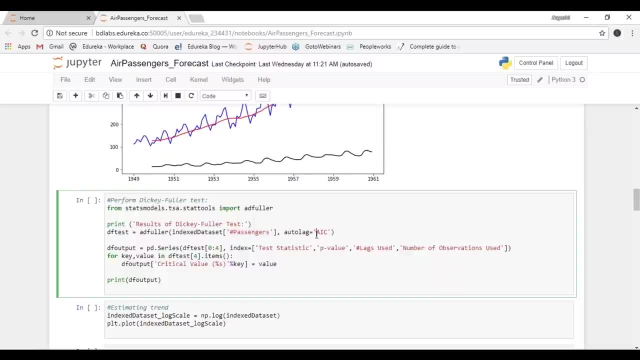 which is the number of passengers, and then I have just given a lag Which is equals to AIC. Now, AIC is basically a chi-k information criterion. Now, what does this AIC mean? So AIC gives you the information about what you wanted in time series. 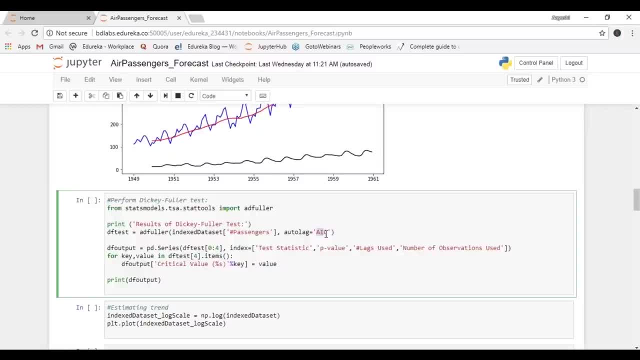 the exact value, of the actual value, and it analyzes from the difference between them. So don't just worry about this, guys, for now. Just think about this as a metric and see what happens when we just run this Dickey fuller test. So when we run, this will have values to test statistics. 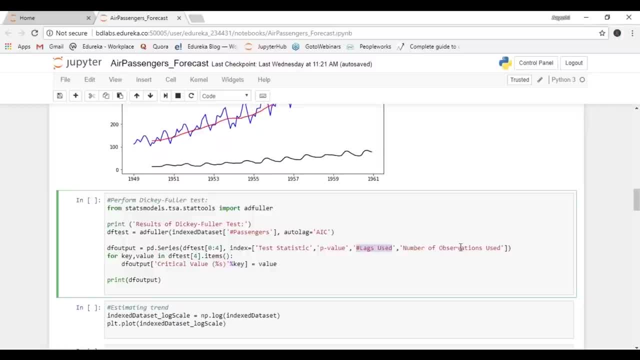 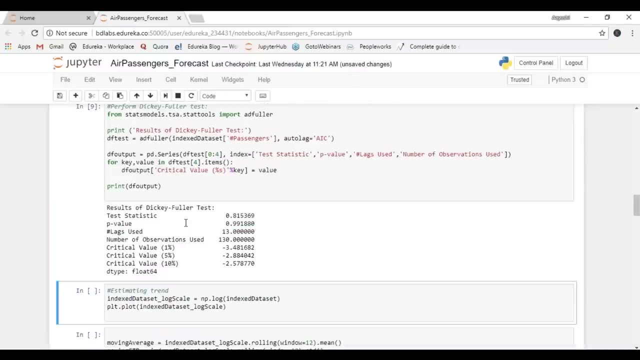 We have t-value- number of lags that has been used and number of observations used- and then we have printed the values in a loop. So now let me just run the cell as well. So this false statement will basically print all the values. Now I have a state statistic value, a p-value- number of lags. 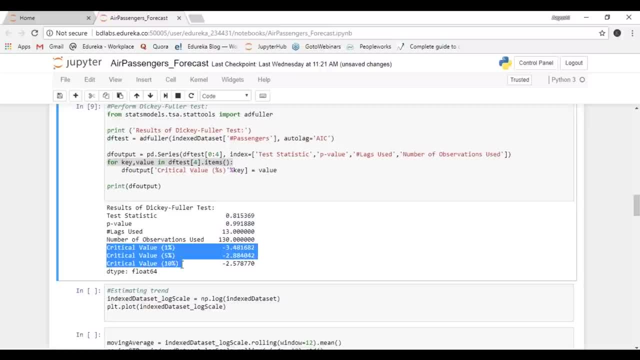 used number of observation and we have critical value at different percentages. So here your null hypothesis says that your p-value should be always less. So here we have a very large value that is 0.9.. So this should be somewhat around 0.5.. 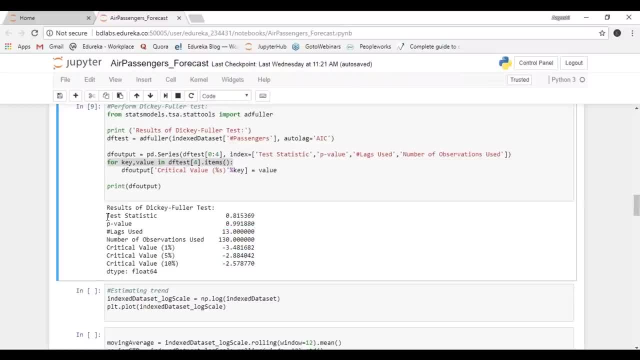 So that would be a great thing. Also, a critical value should also be more than the test statistic. So here we cannot reject the null hypothesis and we can say that data is not stationary, then what we'll do with estimate the trend? So here also with the results of Dickey fuller. 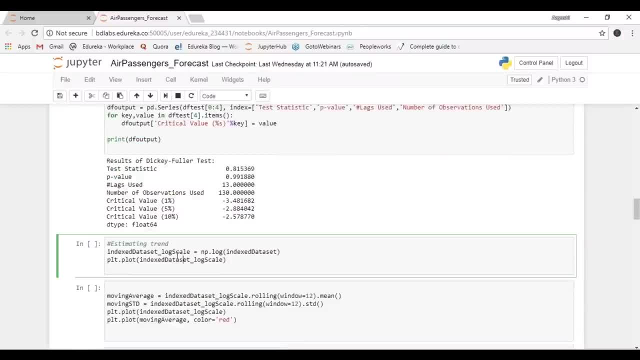 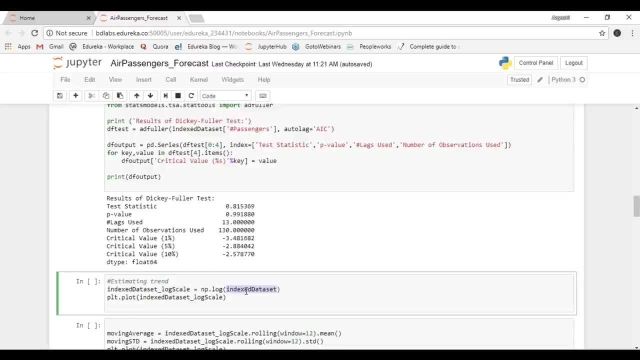 We got to know that the data is not stationary, then what we'll do will estimate the trend. So here what we have done: We have taken a log of the index data set. So index data set is nothing but the data set which has index, has time, or the data. 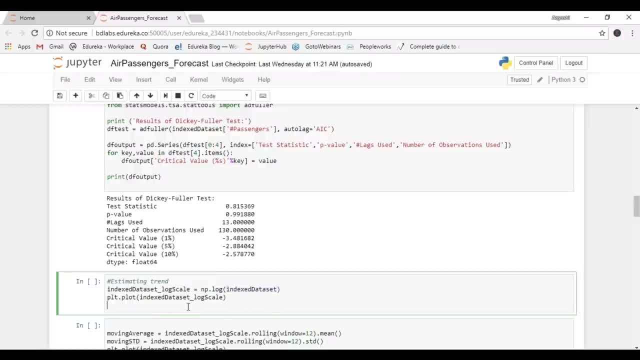 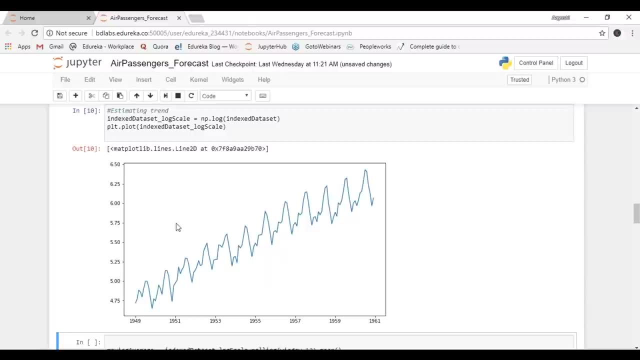 which has been set monthly wise. So here we have just taken a log and let me just run this for you Now. if you see, here numbers on your y-axis have changed because the scale itself has changed. here We have taken the log, but here your trends remains the same. 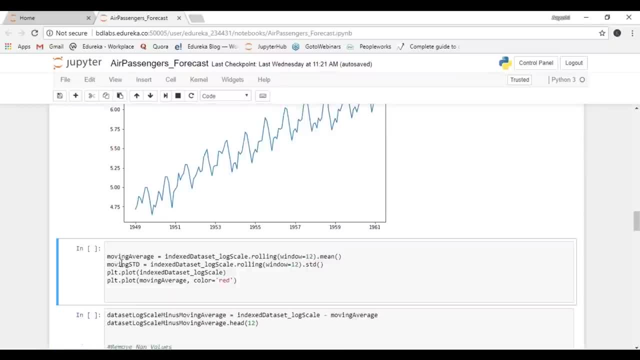 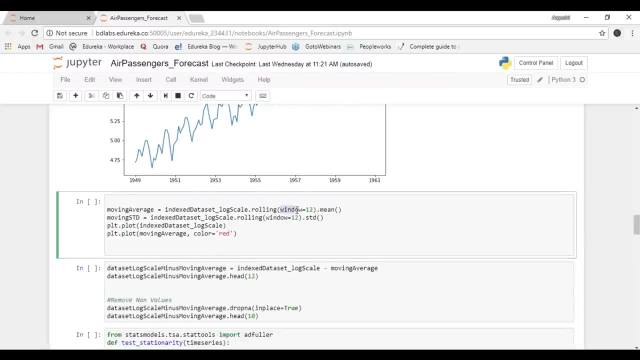 whereas the value of Y has been changed. next, Let us calculate the moving average with the same window. but keep in mind, guys, at this time We'll be taking up with the log time series, So again we'll be having Windows goes to 12. 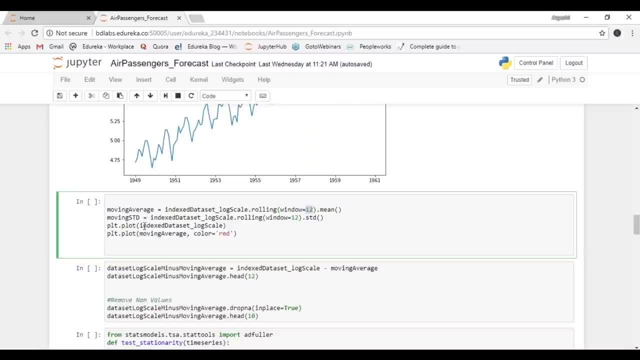 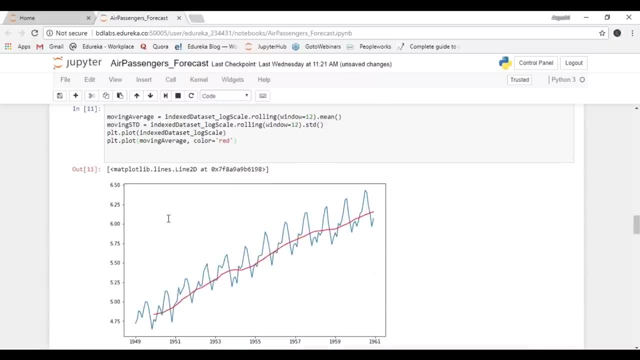 that is nothing but the 12 months, and then we'll be just plotting the graph with the log time series. So here data is already in the log form. So now let me just print it. So here you can conclude: that mean is not stationary. 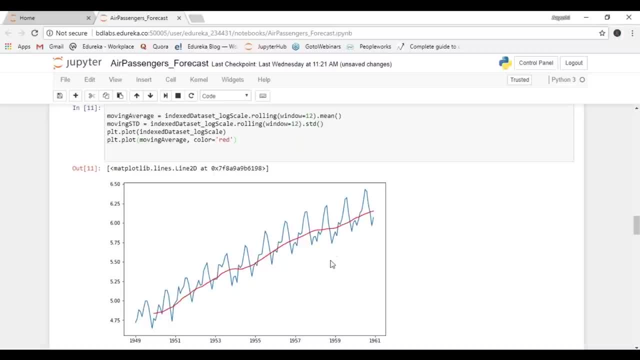 but it is quite better than the previous one. But again it is not stationary because it's moving with the time and this trend is again an upward train, so we can see that the data is not stationary again. Next, what we'll do will get the difference. 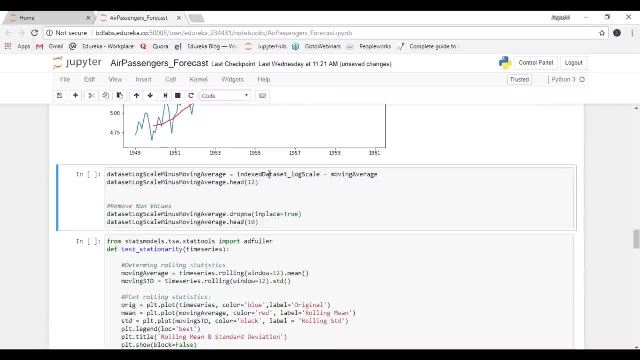 between the moving average and the actual number of passengers. So we have mean and the actual time series. that we have now. why are we doing this Now? The reason is that unless we perform all these transformation, will not get the time series as stationary. 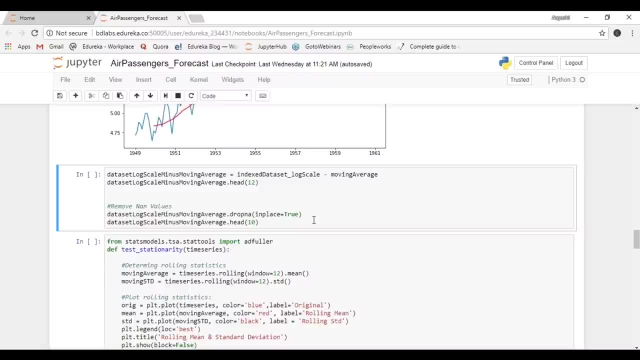 So now you must be having a question as to whether it's the standard way to make a time series stationary. No, it's not, guys, because it depends on your time series, as in how you can make it stationary, Like sometimes, you have to take log. 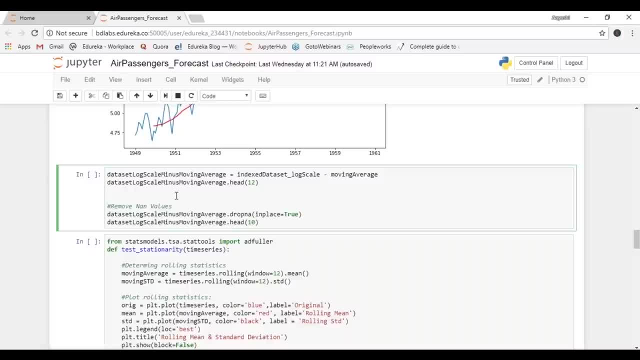 Sometimes you might want to take a square of it Sometime. cube roots. So it all depends on data what it holds. So here we're going to log scale. So we are going to take ma and then subtract both of them. So here we have the log scale and we have the moving average. 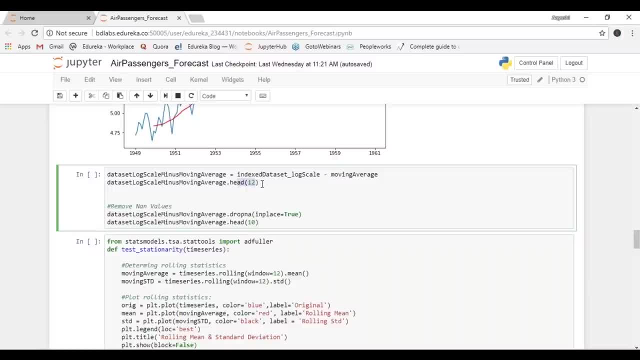 and then we have just printed the head of it. That is the top 12 values. Then what we have done, We have just removed the nan values. So that is done by just typing drop na and the brace. you can write in place: dot, true. 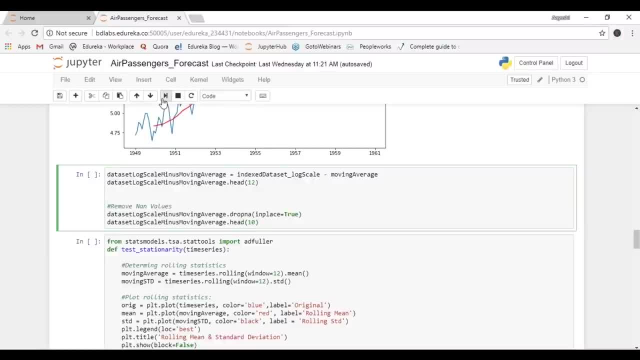 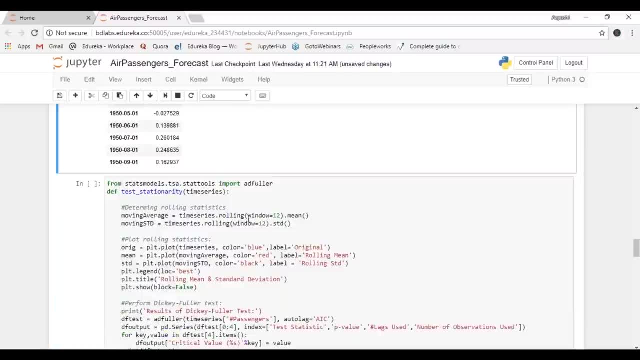 and then just print the head of it. So now let me just run this. So here we have the month and we have the number of passenger, So here we have the numbers, which is basically the difference. then, moving ahead, I have purposely put in actual code of this ADCF test. 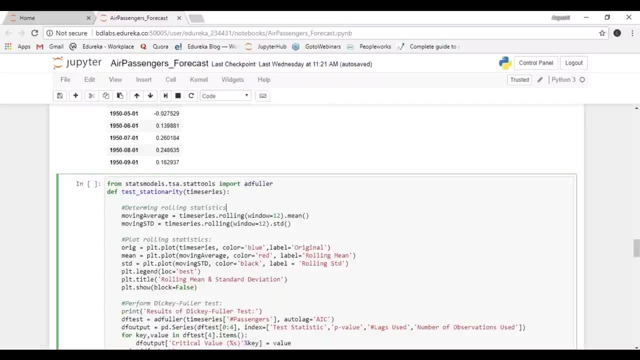 So ADCF, This is augmented Dickey Fuller test. So above I have just applied a simple ADCF function, but this is the whole code, guys. So you have to perform this whenever you have to determine whether time series is stationary or not. 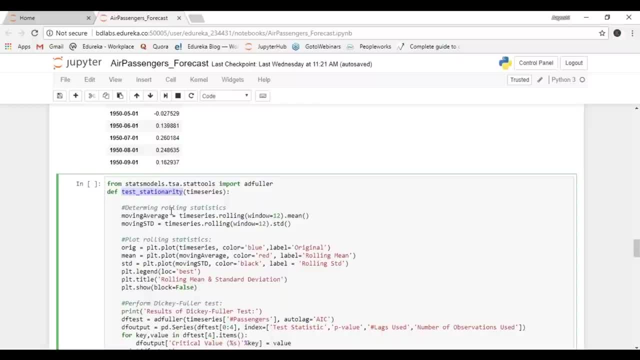 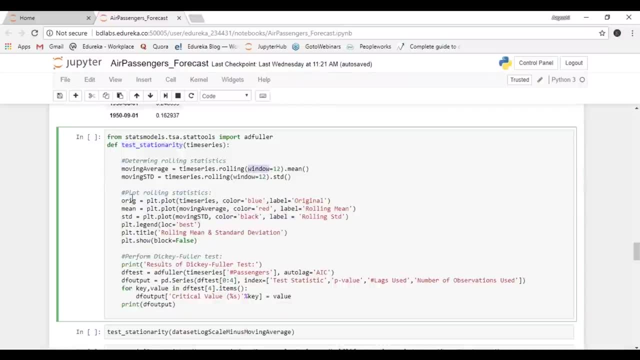 So here I have defined a function which is test stationary, and I have performed both the test. I have determined rolling statistics as well as perform Dickey Fuller test over here I have used the Windows 12 and then I have plot rolling statistics as well. 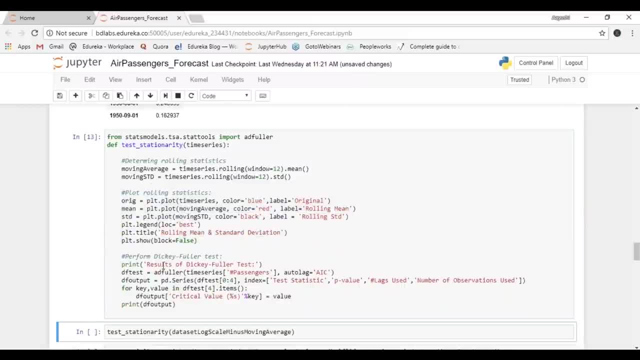 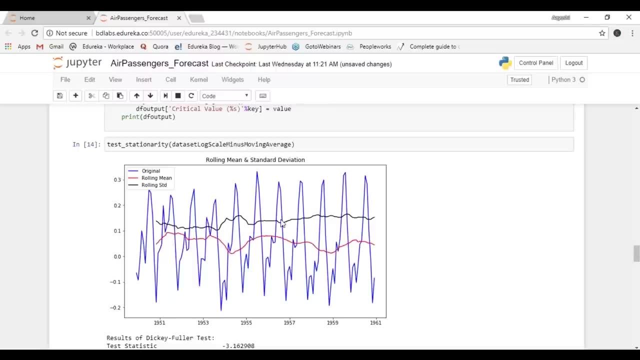 I have performed the Dickey Fuller test as well, So let me just run this and I'll just run the function as well. So now, if you see you have the original data as blue lines, then you have standard deviation in black line and you have rolling mean in red line. 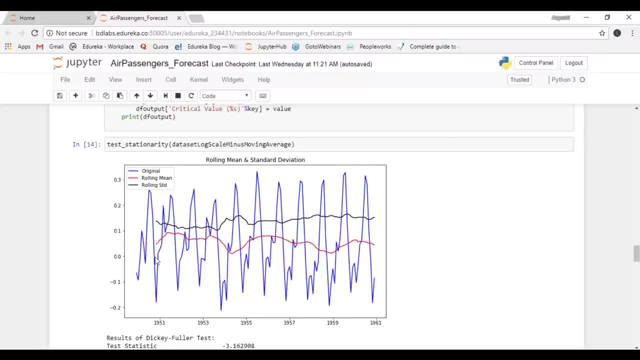 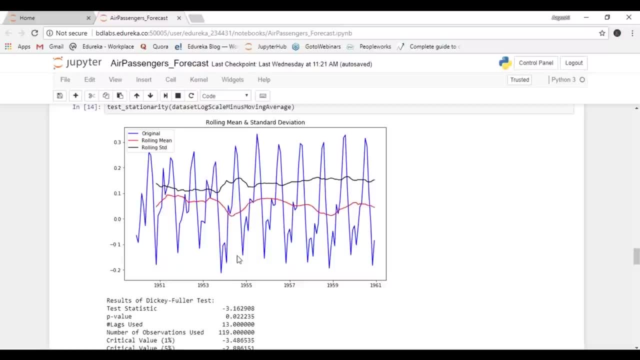 So here you can visually notice that there is no such trend, or you can say it is much better than what we used to see earlier. So here we have rolling standard deviation and we have rolling mean. now let me see the ADCF results as well. 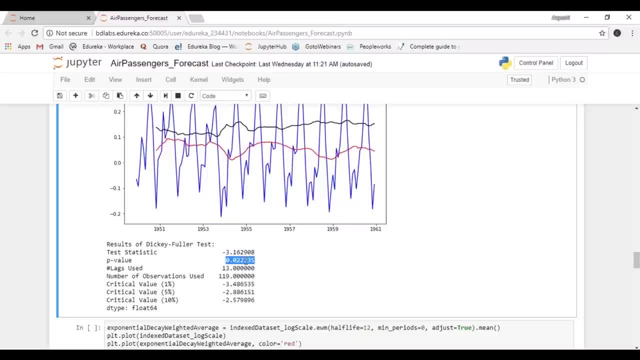 So here, if you notice, your p-value is relatively less. in early cases we used to have 0.9 something, and over here You have p-value at 0.02.. Now, if you notice your critical value and your test statistics value is almost equal. 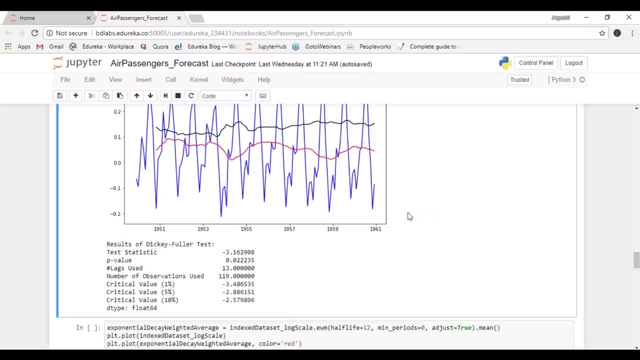 which basically helps you to determine whether your data is stationary or not. So I hope by now you got the idea, between the Dickey Fuller test and the rolling statistics test, as to how you can determine whether the data is stationary or not. next, what I have done. 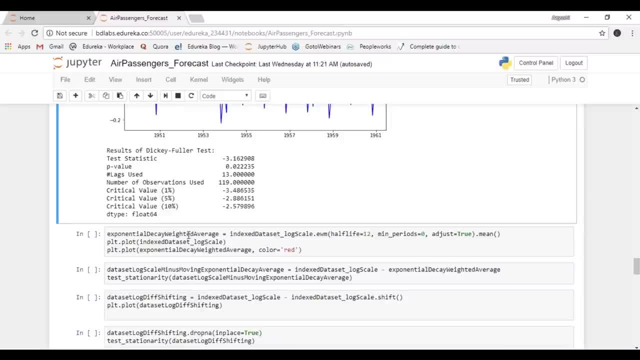 I've calculated the weighted average of time series. Now, why I have done this? because we need to see the trend that is present inside the time series. So that is why we have calculated the weighted average of time series. So now let me just run this. 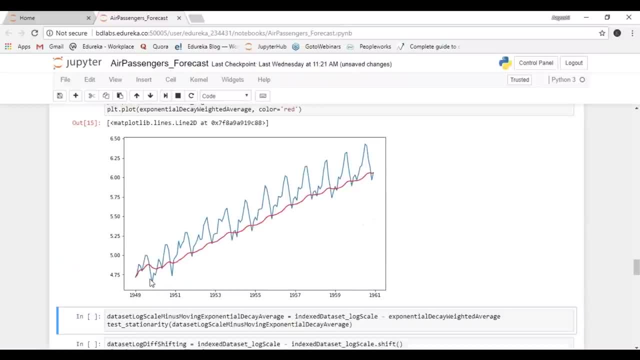 and you'll get to know why I'm talking about this. So, as you can see here, as the time series is progressive, the average is also progressing towards the higher side. So here your trend is upward and keeps on increasing with respect to time moving ahead. 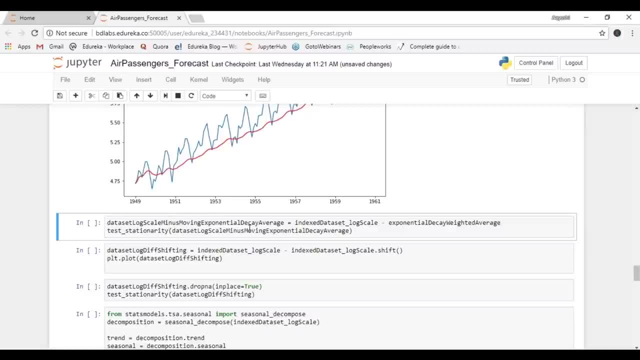 Let's see another transformation where we have a log scale and then we subtract the weighted average from it. So in a previous scenario we have subtracted simple mean, but in this will be using weighted mean and then we'll check for stationarity. So here we have just subtracted them. 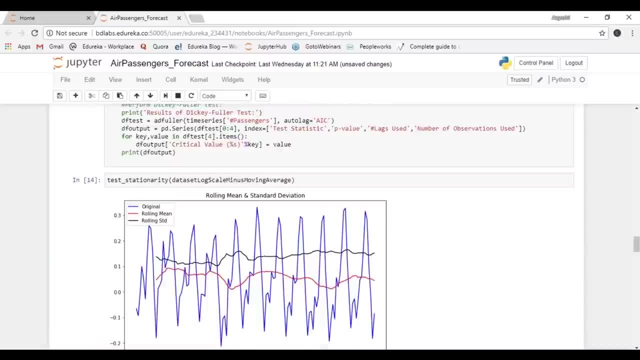 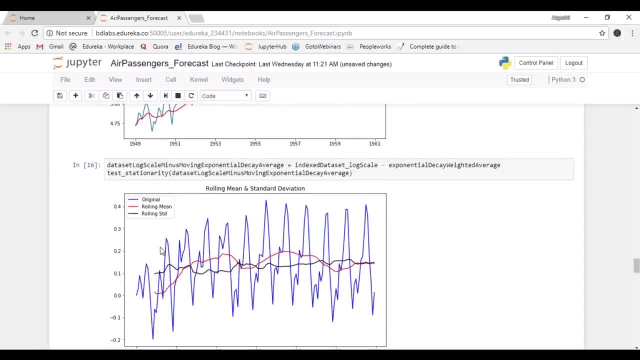 and then pass the variable in the test stationarity function that we have just defined it over here. So over here it will go through both of the tests and then it will display the results. So over here I'll just run the cell. So over here you can notice. 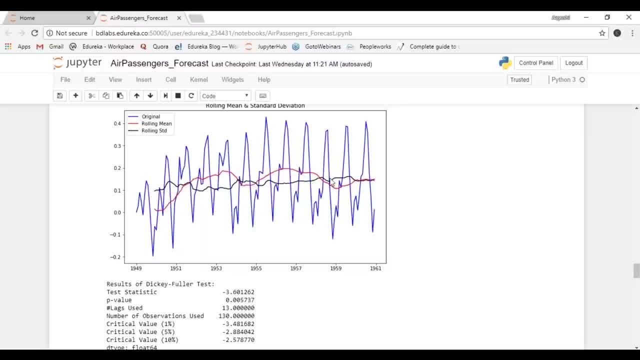 that your standard deviation is quite flat. It is not moving here and there. In fact, you can also say that this doesn't have any trend. Also, we notice the rolling mean. it is quite better than the previous one. Now let me just see the results of ADCF test as well. 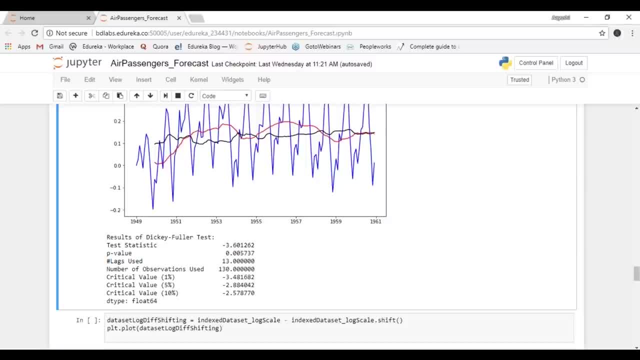 So over here you have a very less value of P. that is, P is equals to 0.0.. 0.05.. So your TS is again stationary, which means that your time series is again stationary. So here you can use both this transformation. 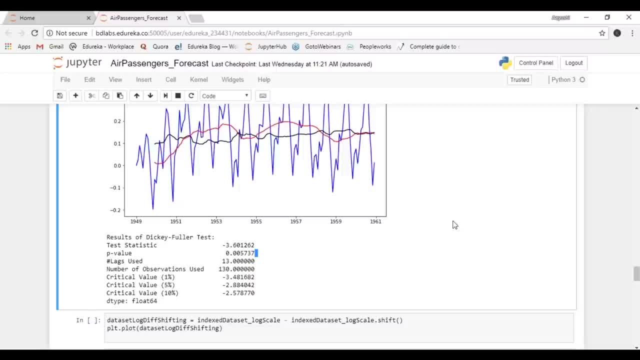 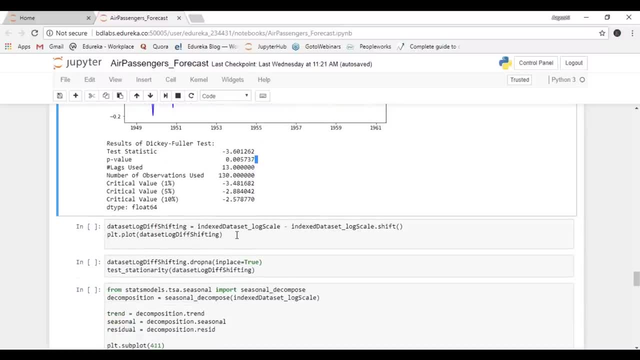 to check whether your data is stationary or not. So now we know that our data is stationary. Now what we'll do will shift the values into time series so that we can use it in the forecasting. So what we have done earlier: we have subtracted the value. 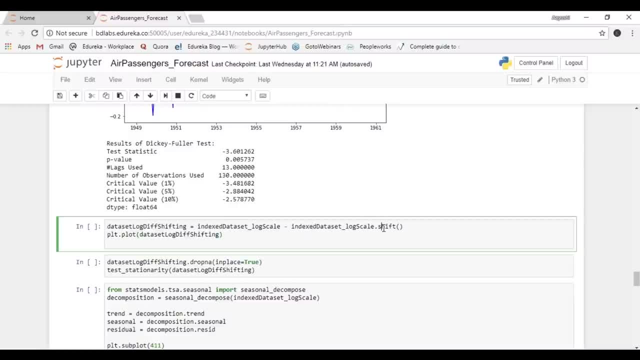 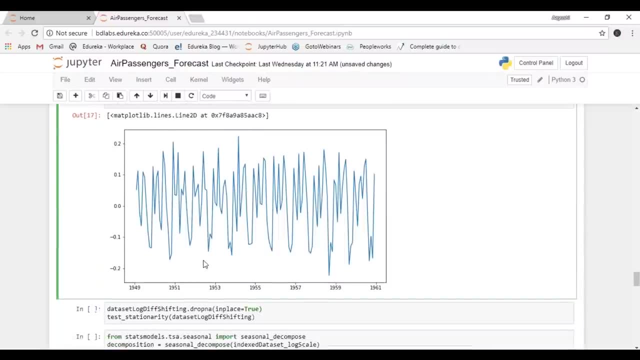 of mean from the actual value. Now, what we'll do? we'll use the function called a shift to shift all of those values. So here let me just run this plot. So this is how the plot looks like now. here We have taken a lag of one. 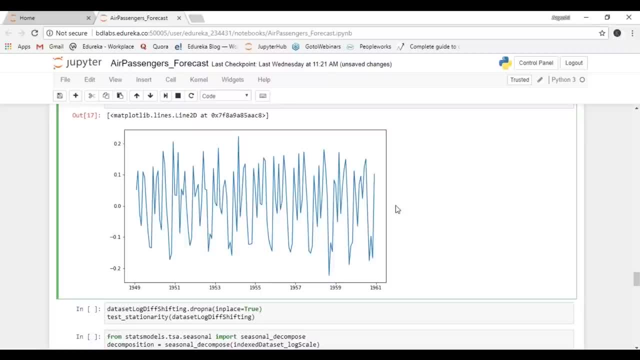 So here we have, just shift the values by one, or you can say different your time series once. so, guys, if you remember, I talked about the Arima model. So Arima model has three models in it. That is the AR model, which stands for autoregressive. 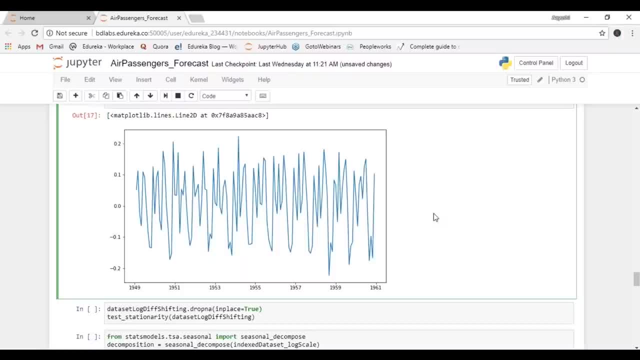 Then we have ma model, that is for moving average and eyes for the integration. So Arima model basically takes three parameters and D there stands for the integration part. or you can say how many times you have differentiated a time series. So here your value becomes one. now next, what I have done. 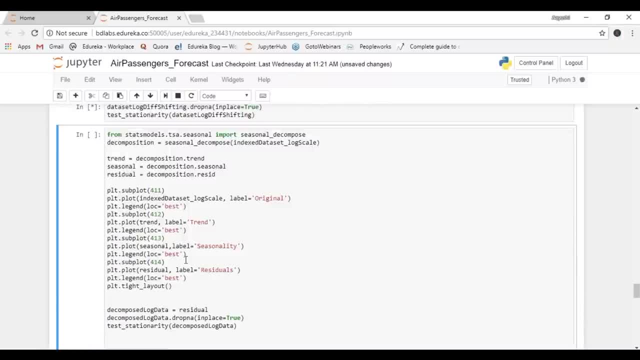 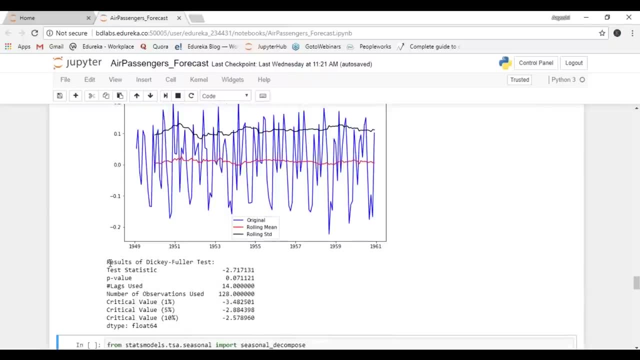 I have simply dropped the nan values. So here, if you just run this code, you'll see that output is quite flat. So here your null hypothesis, or the augmented Dickey fuller test wherein will take the null hypothesis, is rejected, and hence we can say that your time series is stationary now. 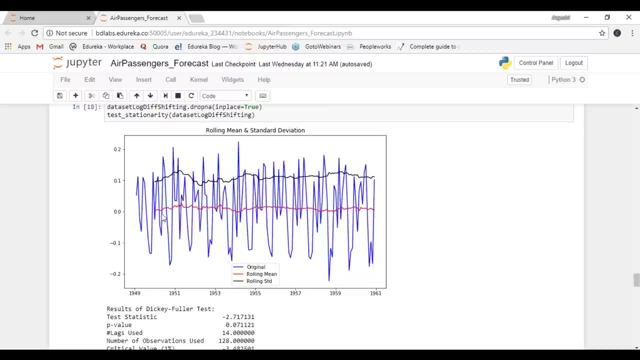 So here you can say that you again have blue as the original data, you have red as your rolling mean and you have black as your standard deviation. So visually also we see that there is no trend present and it's quite flat. So here we can say that your time series is stationary now 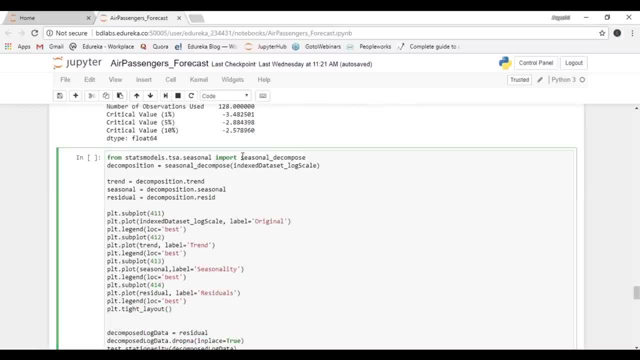 let us see the components of time series. So here you first need to import from stats model to TSA dot. seasonal input, seasonal decompose. So here, your seasonal decompose segregates three components, that is, trend, seasonal and residual. So here what we have done. 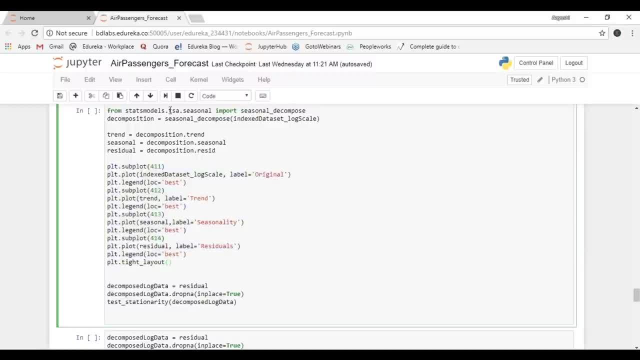 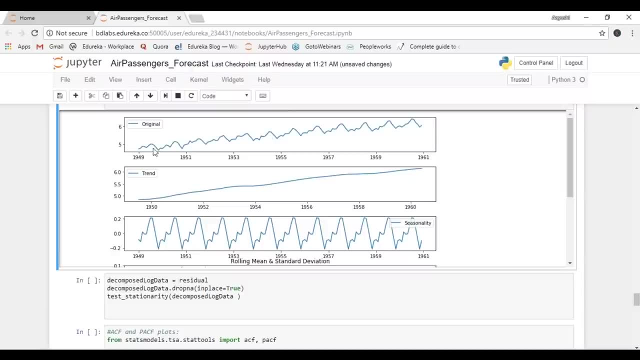 We have simply plotted these graphs and let us see how all these graphs looks like. Let me just run this, So this is how your output look like. this is my original data, which we saw that there was a trend, So this is my trend line. 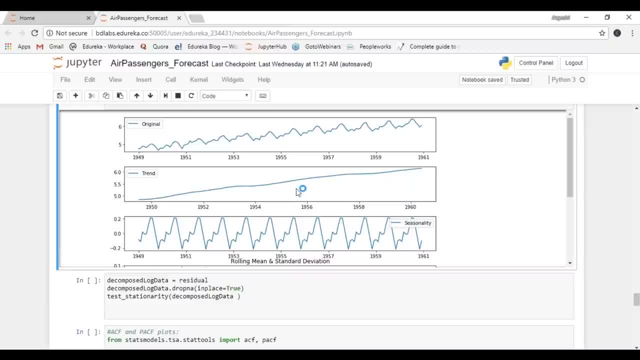 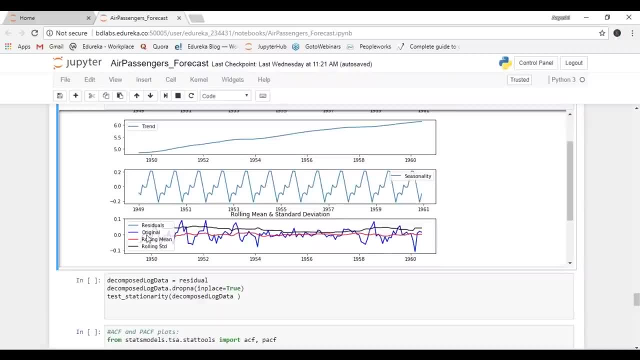 So this is going upward in which you can say it's quite linear in nature. along with that, We have seasonality also present in high scale, So we have a seasonality graph over here, and then we have the residuals as well. So residuals are nothing, guys, the irregularities. 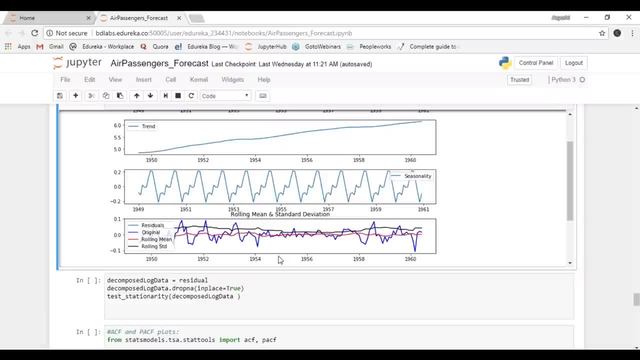 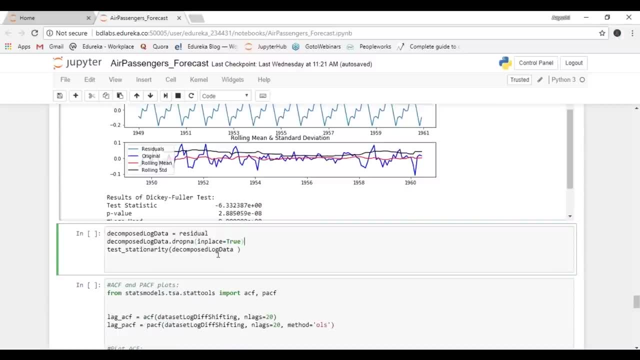 that is present in your data. So they do not have any shape, any size, and you cannot find out what is going to happen next. So it's quite irregular in nature. Now, what we are going to do, we'll check the noise if it's stationary or not. 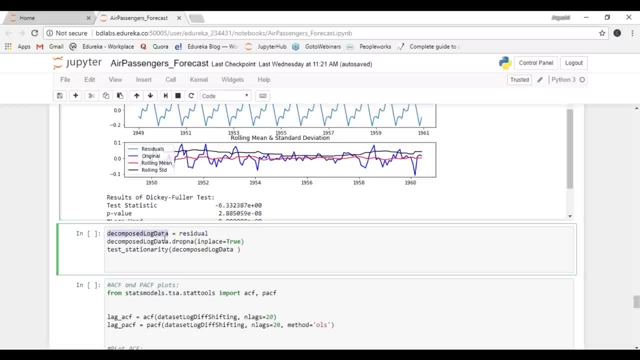 So over here we take the residual and we'll save it in a variable that is decomposed log data and again I'll just pass it to the same function that we have just created above, which is test stationary. and inside this test stationary function We have to test, that is, rolling statistics and ADCF test. 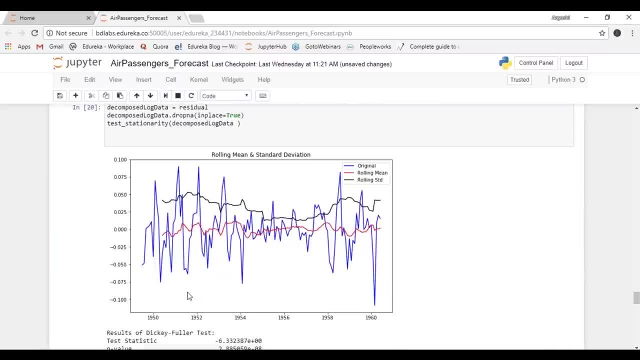 So now let me just run this cell and this is how your graph looks like. So, looking at the output visually, you can say that this is not stationary. That is why we have to have your moving average parameter in place, so that it smoothens it out to predict. 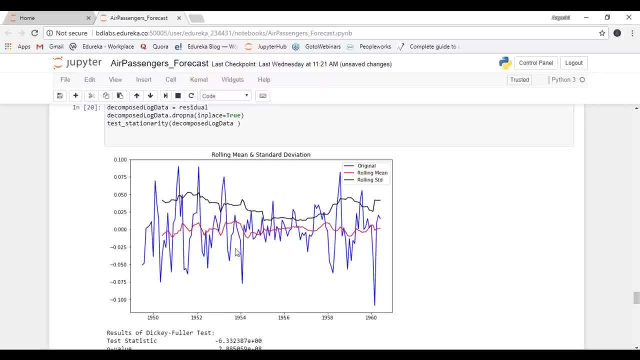 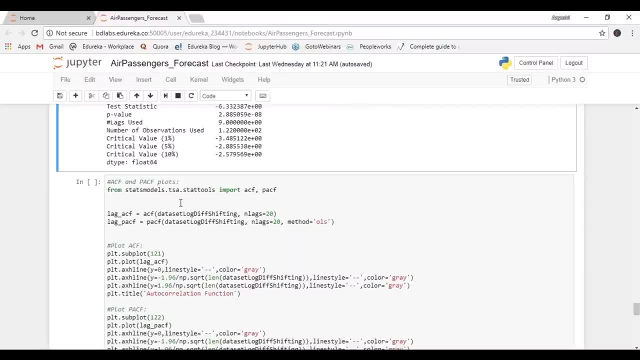 what will happen next? now we know the value of D, but how can you know the value of P and Q, that is, the value of autoregressive lags and the value of moving average? So here, as I told you guys, we need to plot ACF graph. 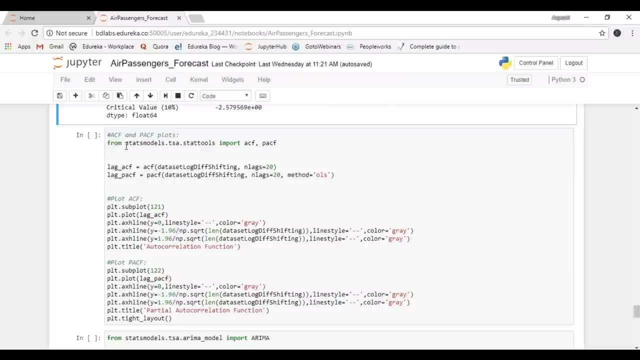 and PCF graph. So in order to calculate the values of P, we need to plot PCF graph and in order to calculate the value of Q, We need to calculate ACF graph. So ACF basically refers to your autocorrelation graph and your PSCF stands for partial autocorrelation graph. 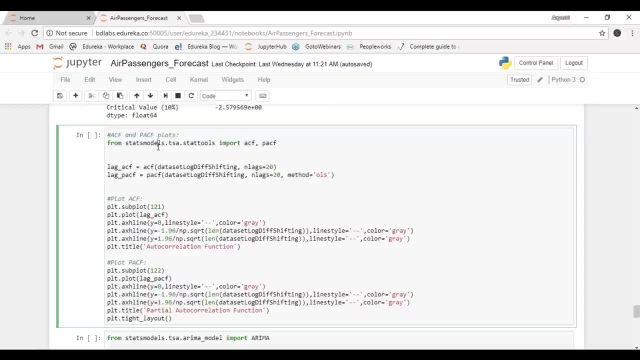 So in Python we first need to import these two graphs, that is, from stats model, dot, TSA, dot, stat tools, import ACF and PCF. then, using this function- ACF and PCF- We are just passing a data set and we have preferred a method that is OLS. 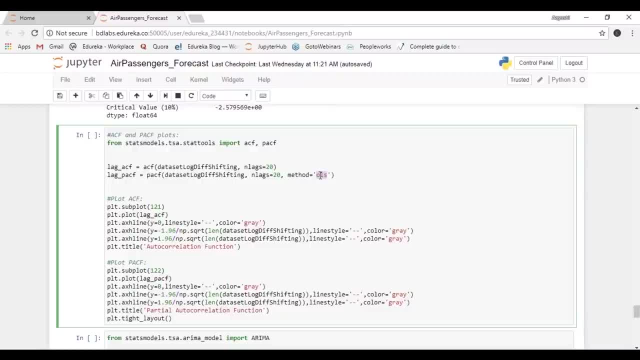 So there are various methods, but we usually prefer OLS. OLS is ordinary, least square method. Then what we have done? we have simply plot ACF graph and we have plotted the PCF graph. So now let me just run this and let's determine how you can calculate P value and Q value. 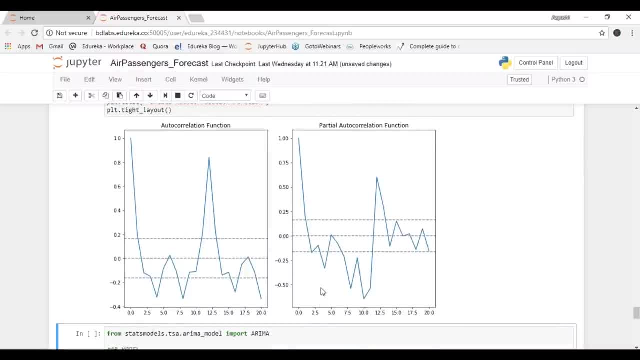 So, guys, this is my autocorrelation graph and this is my partial autocorrelation graph. now, in order to calculate the P and Q values, You need to check that. what is the value where the graph cuts off it? or you can say, drops to 0 for the first time? 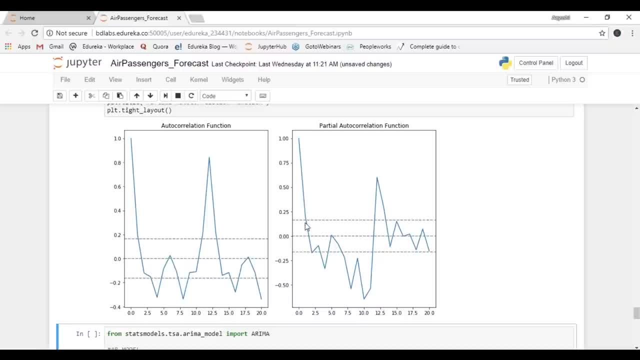 So if you look closely you have it touches the confidence level over here. So here if you see your P values almost around 2, and similarly, if you look at this graph, you'll see that it cuts it over here or drops to 0 over here. 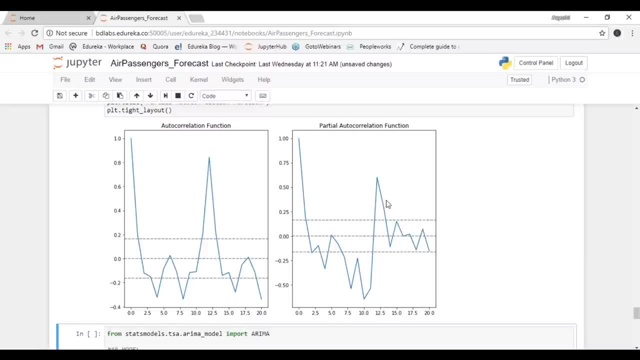 and then the value of Q also becomes 2.. So this is how you can calculate the value of P and Q using PCF graph and ACF graph. next, We have the value of P, We have the value of Q and we have the value of D. 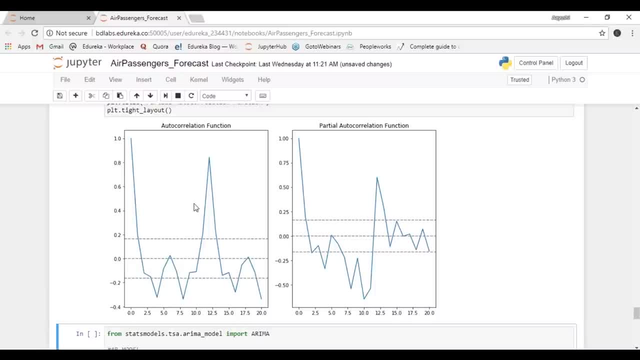 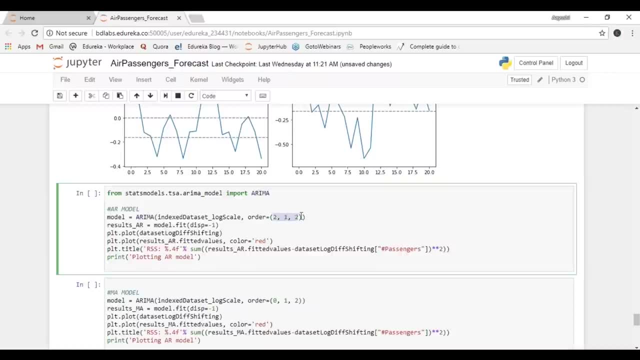 So what we can do. we can simply substitute these values in the Arima model. So here what I have done. I first imported the model Arima and then, using the function Arima, I have the order listed over here. So I have P value as 2. I have different set one. 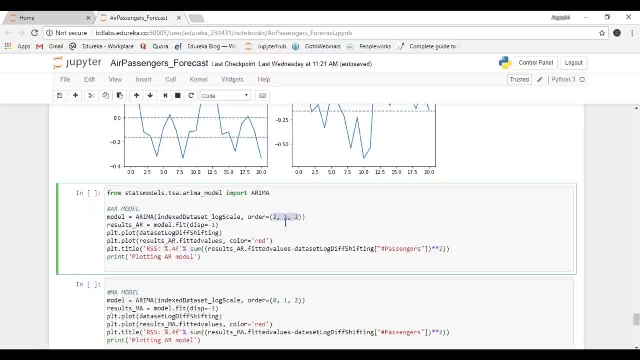 So my D value, It becomes 1, and my Q value is again 2.. So here I have just plotted the graph and then calculated the RSS, which is the residual sum of squares. So here let me just run this graph. So here you can see, the residual sum of square is quite good. 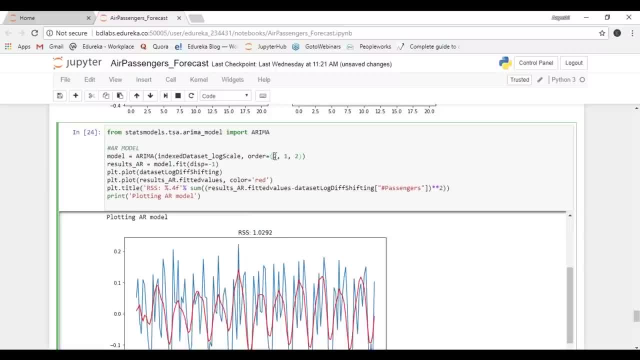 That is 1.02.. So here you have plotted the values of P, Q and D as 2, 2 and 1. now you can also play around with these P and Q parameters. Now let's say I want to change the parameters to 2, 1, 0.. 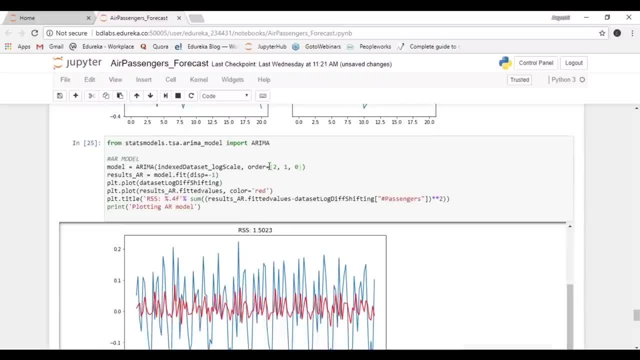 So if I do that, let me just run this again. So here, if you see, once I have just changed the value to 2 1, 0, my RSS score has been increased. So greater the RSS, the bad it is for you. Now let me again change it to 0, 1, 2. now, in that case, 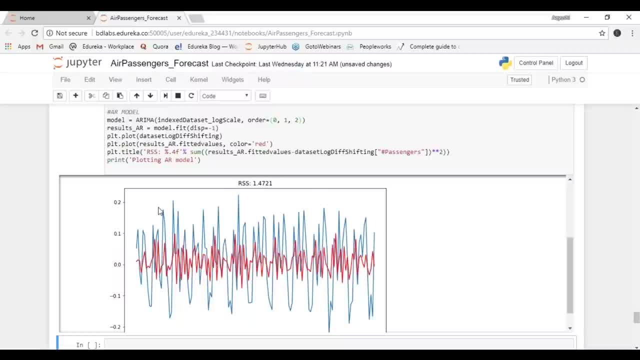 Also, my RSS has been increased to 1.4.. So here you need to take care of the RSS part. So the greater the RSS, the bad it is for you. So here we'll just revert back to 2, 1, 2, wherein we have the value of P as 2, Q as 2. 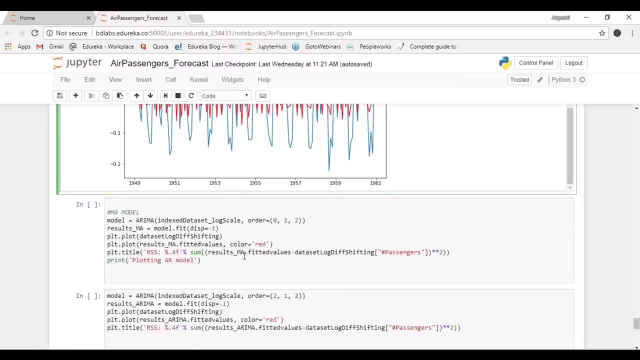 and we have taken only one difference, So the value would be 1. now let's take the moving average model in consideration. So here a p-value is 0. now for our model. You have to do 2, 1, 0. next for AR model. 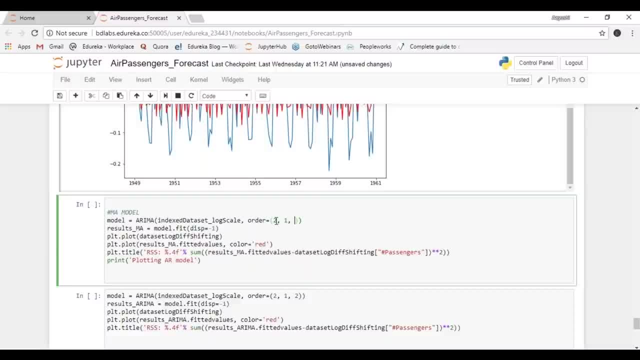 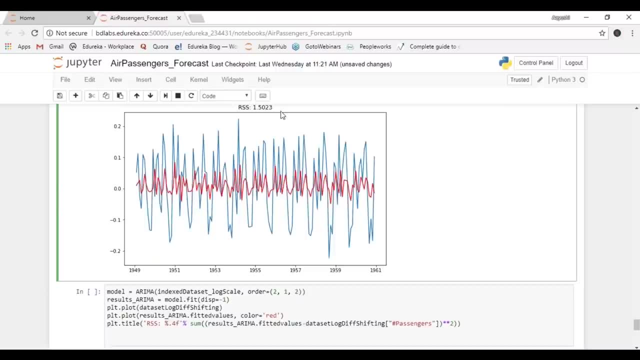 What you can do. you have to do 2 1 0, wherein you have the value of Q as 0. So here I have 2 1 0 and let me just run it for you. So here you can see that your RSS has again reach 1.5.. 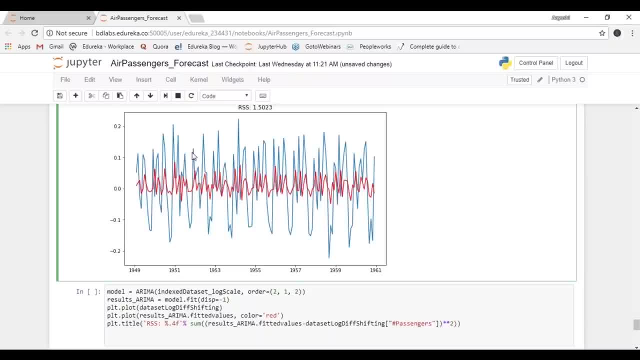 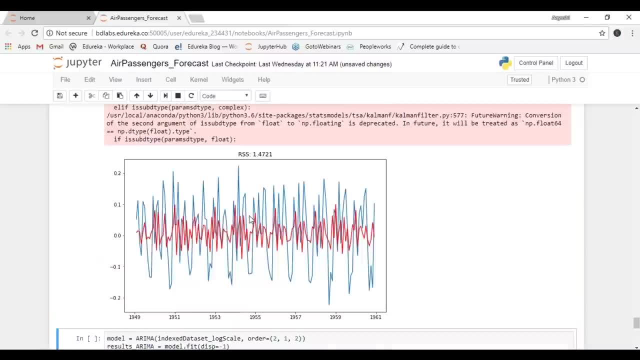 Now we have seen that with respect to AR, that is, your autoregressive part, your RSS is 1.5. now offer again. go to ma, wherein I have the values as 0, 1, 2. the RSS score is 1.4.. So here we conclude that with respect to autoregressive part. 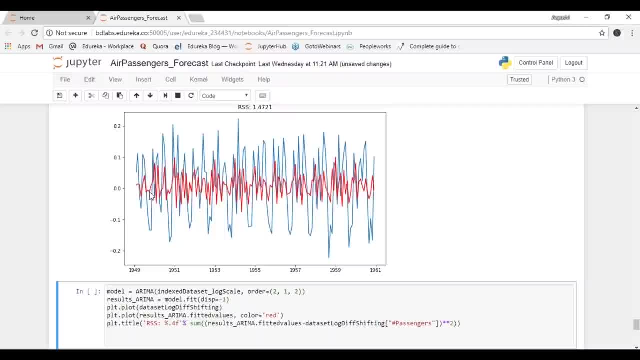 We have the RSS as 1.5 with respect to moving average. We have the RSS is 1.4 and if we combine both of them and make Arima out of it, that is this part. that is 2 1: 2. we have very less RSS. 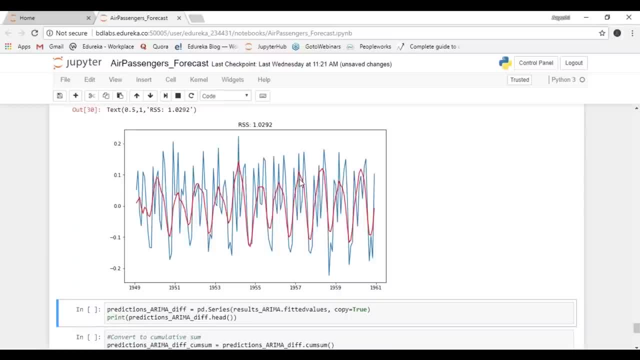 So it may just run this as well. So here, when I substitute the values as 2, 1, 2, that is P, and Q value is equals to 2 and D we have taken as one. So here your Arima model gives you RSS of 1.02,. 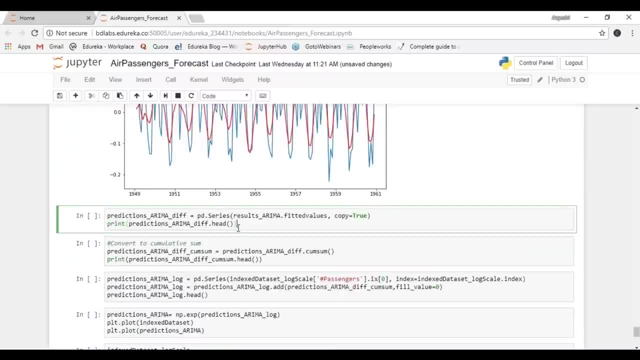 which is quite good. next, what we'll do? Let's fit them in a combined model, that is Arima. So here we have seen that, with respect to AR, we have RSS is 1.5. with respect to ma, that is moving average- We have RSS as 1.4. 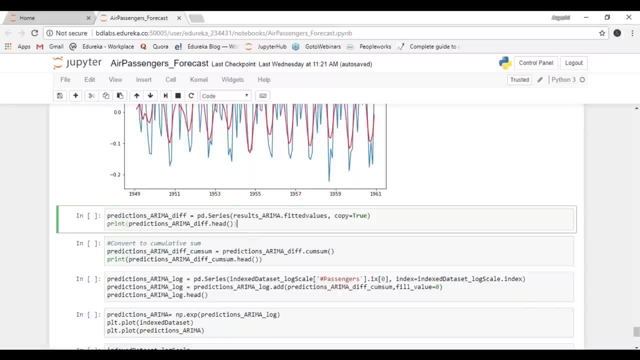 and when we apply the combined model, that is, Arima, the RSS, or you can say, the residual sum of Square is dropped to 1.02.. So here let's do some fitting on the time series, on what data we have. So here we have just converted the fitted values. 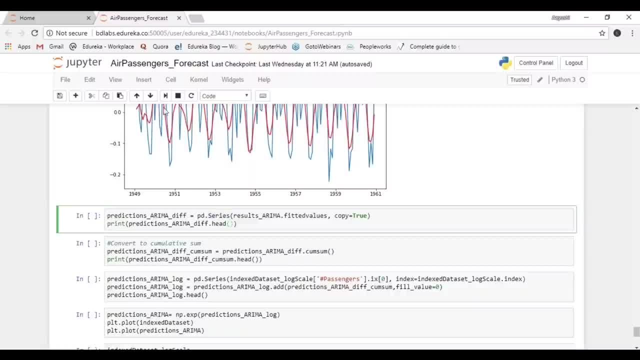 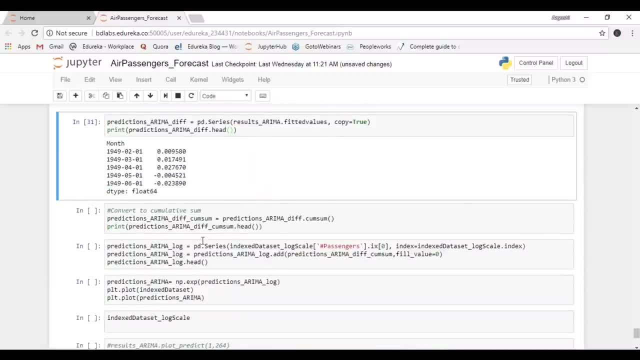 into a series format and then we have just printed the head of it. So now let me just run this over here. We have the month as well as the predictions over here. next, what we'll do will find it, the cumulative sum, and then we'll find the, and then we're going. 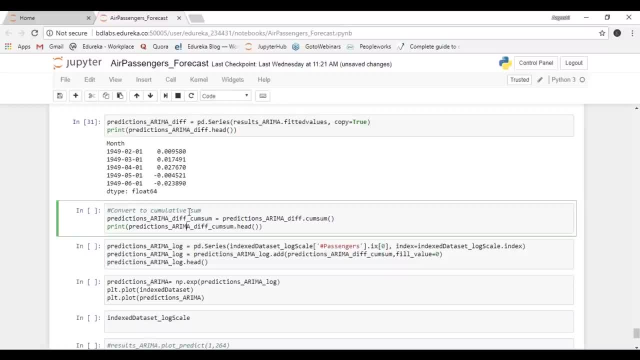 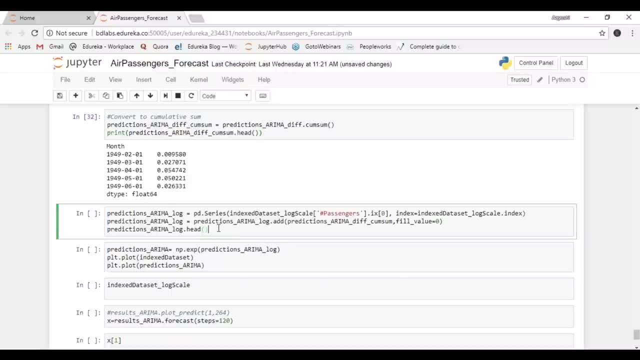 to have the predictions done for the fitted values. So now to calculate the cumulative sum, We have the function called as cum sum and then again we have just printed the head. So this is my result and finally, we're going to have the predictions done. 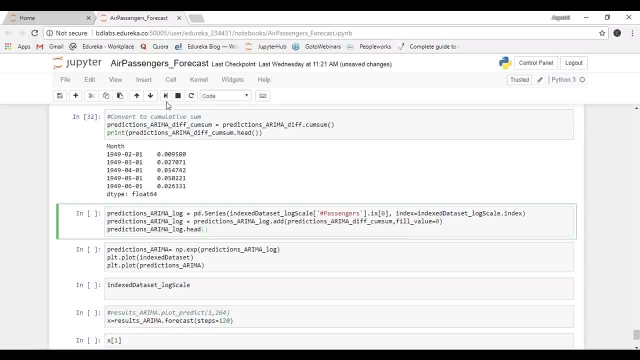 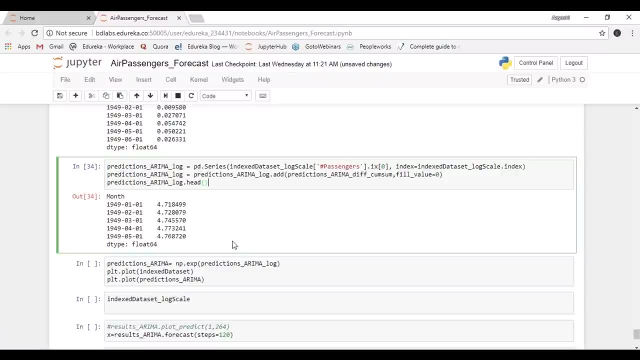 for the fitted values, and then we have just printed the head of it. So now let me just run this next. We also keep in mind that after performing these transformation, We also need the explanation of the whole data, so that it comes back to the original form. 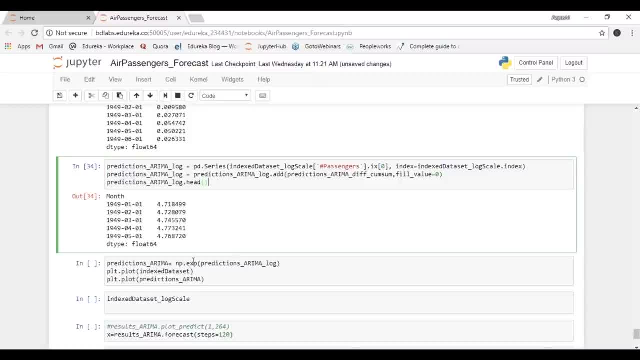 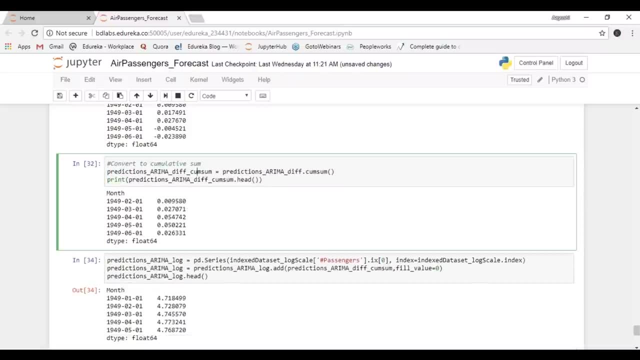 from where we have just started using it. So in order to know the values in that form, you need to take the exponent of it. So these are the three steps which are very important for data transformation. So you'll be finding cumulative sum will do the predictions. 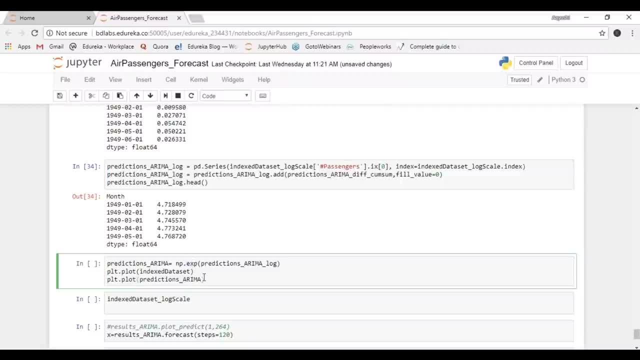 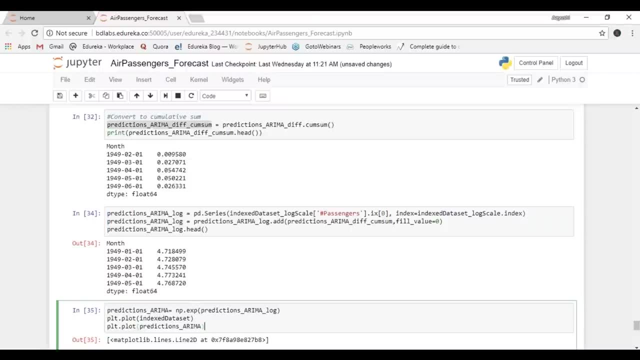 and will and will also calculate the exponent of it, So as to get your data in your original format now. after that, we just plot the actual values to how our model has fitted. So now let me just run this So you can see that the orange line is basically the model. 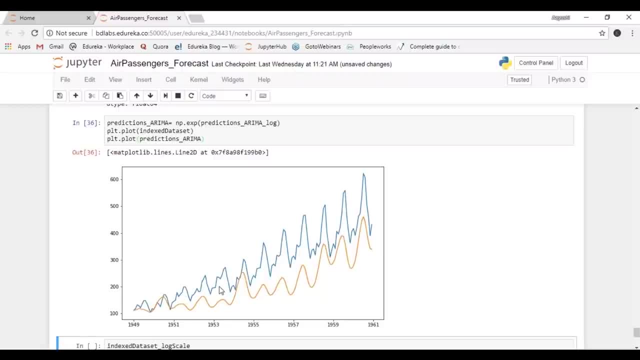 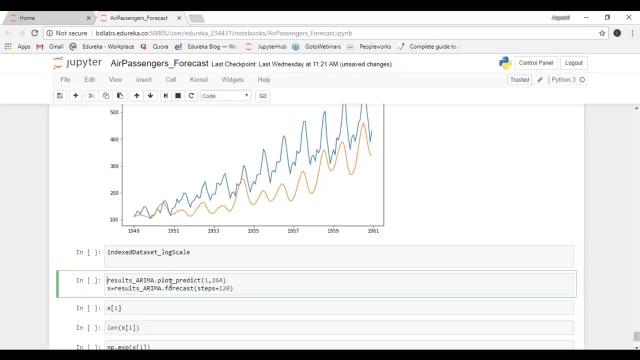 that we have fitted, and here you can see at only the magnitude is wearing, whereas the shape has been properly captured by the Arima model. Now how we can do predictions, guys. now there is a function in Python that is predict now before predicting the values. 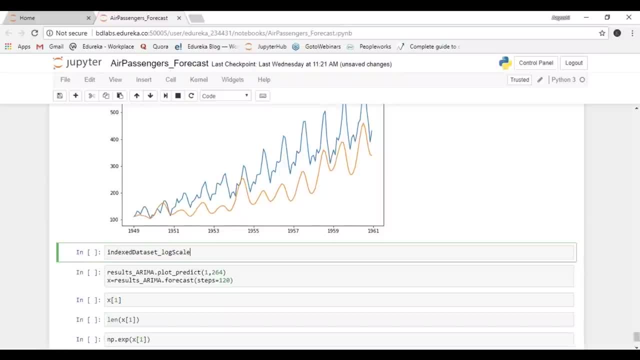 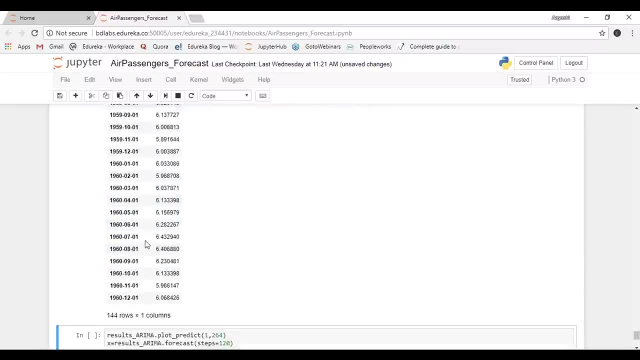 Let me first see my data. that how many rows are there in my data set? So this is my data set name. So now let me just run this. So here we have the data set from 1949.. We have the number of passengers. it will go on to 1960. 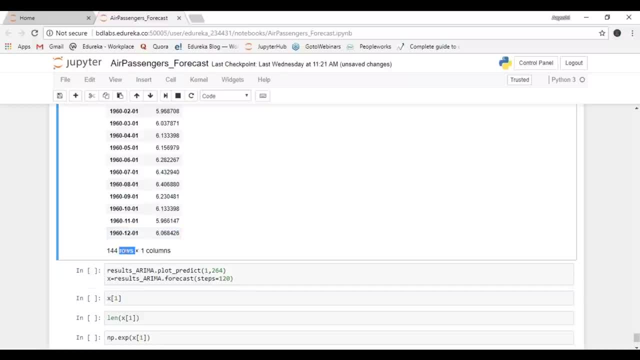 and we have 144 rows into one column. So here we got to know that we have 144 rows. So what if I want to predict it for next 10 years? So what will be my prediction? now here you have to see that. how many number of data points would you want? 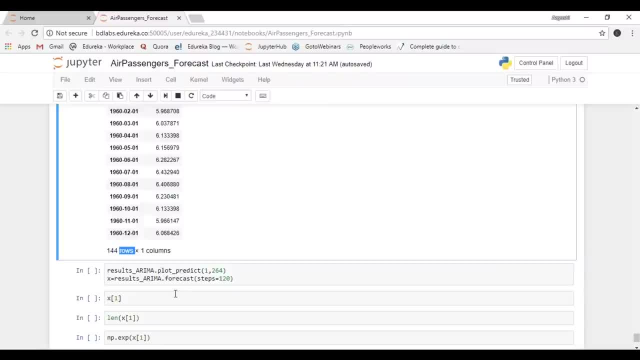 So let's say, if you want to predict for 10 years, So the number of data points would be 120. that is 12 into 10.. So here, if you want to predict it for 10 years, you have 120. so using that plot, dot predict function. 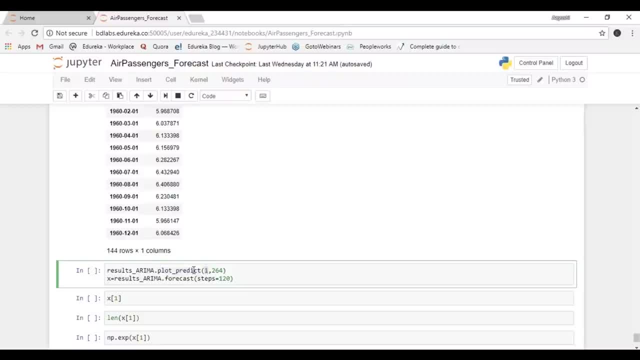 I can actually predict the future. So here, using this function, I'll give the first index of the time series and then the number of data points you want the time series for. so I have 144 rows plus 120 because I want it for 10 years. 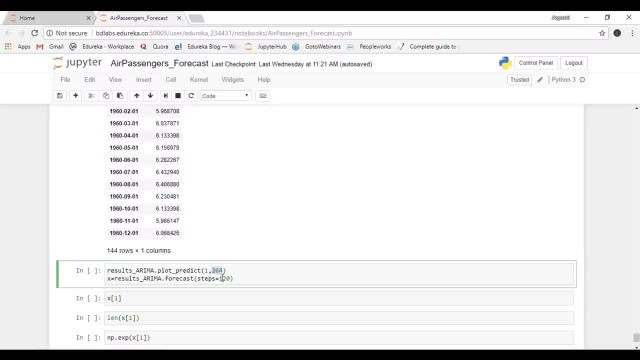 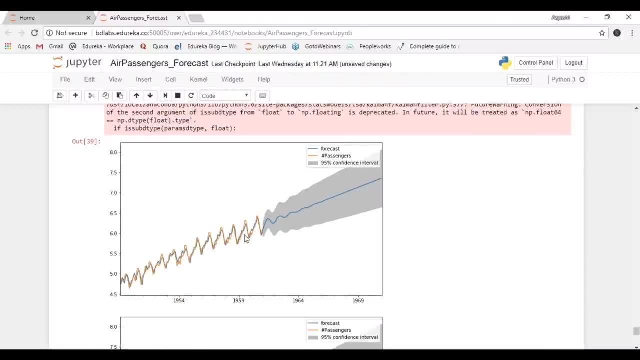 So 144 plus 120 is equal to 264.. So I'll write it over here Now. let me just comment this for now and let me just run it So over here. if you can see, the blue is the forecasted value and this gray part is your confidence level. 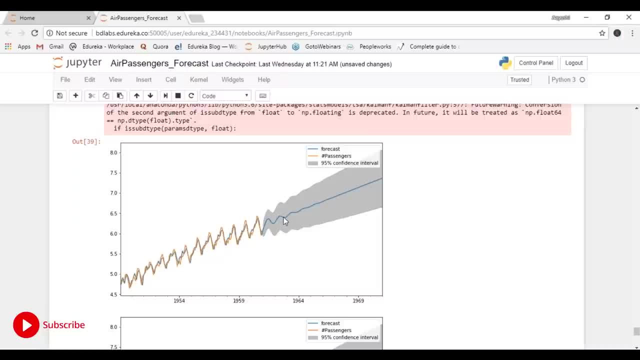 So now, whatever happens or however you do the forecasting, this value will not exceed the confidence level. So this is how you can see that for the next 10 years You have the prediction somewhat like this. So this is how you can do prediction. 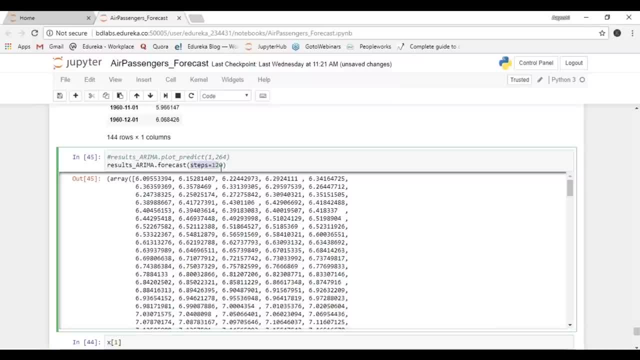 and if you don't want to see the graph, you can actually write in the data point. So here I want the prediction for 10 years, So I have just type in the steps. that is equals to 120 and you get the result in an array format. 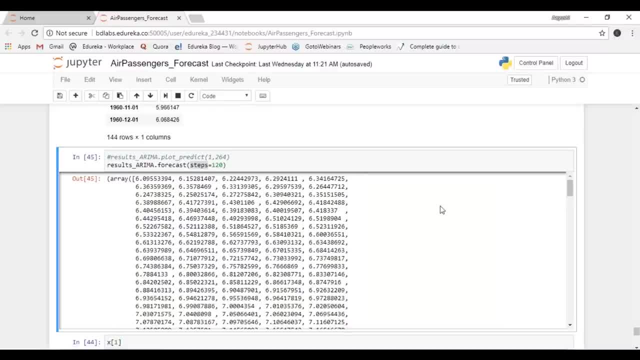 So that is how you can perform a lot of operations with this data and predict it for, let's say, six months, 12 months, next year, 10 years, and it's totally up to you guys. Whatever topics that I've covered, I hope these are clear to you. 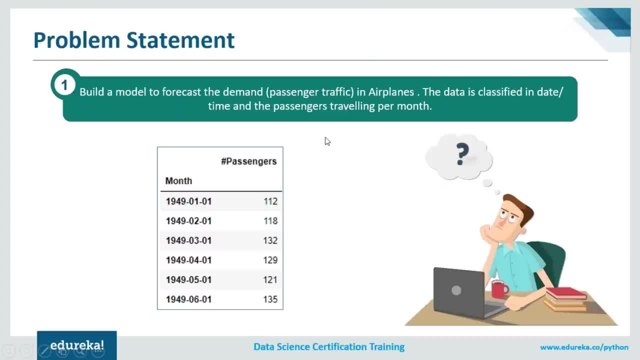 So now let me just go back to a presentation and let's see what all we are left with. So here we have just build a model wherein we have forecasted the demand for the next 10 years. So in a data set we have the date in the monthly basis. 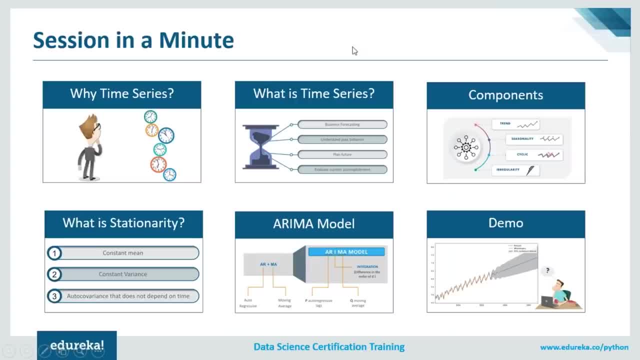 and we have the number of passengers. So that's all for today, guys. Now let me just recap what all we have covered till now. So we have started off by discussing what exactly is time series, and we've also gone to the various components.